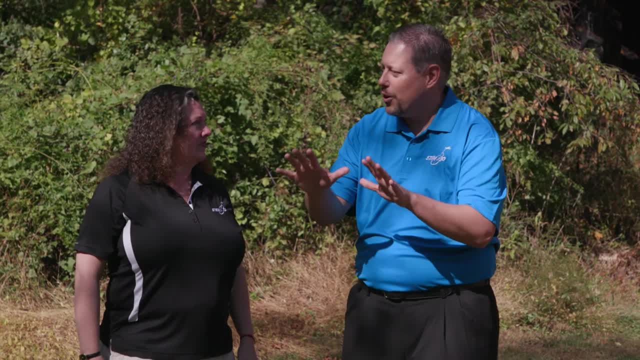 I knew you were going to say that We're going to learn all about simple machines, even the ones we use at the National Air and Space Museum, But we're going to start by looking at a mill. Let me introduce you to a friend of mine, Catherine. 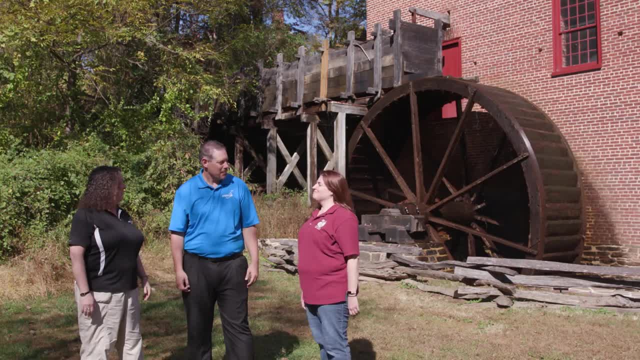 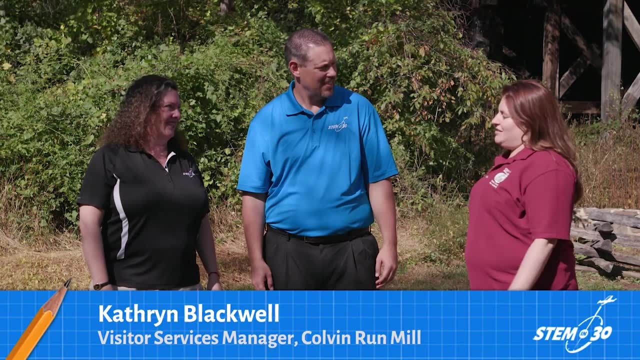 Beth, this is Catherine. Hi, Catherine. So we're here at. Welcome to Colvin Run Mill. Do you want to tell us a little bit about the mill? So we are a 19th century grist mill and we still grind grain today the way they would. 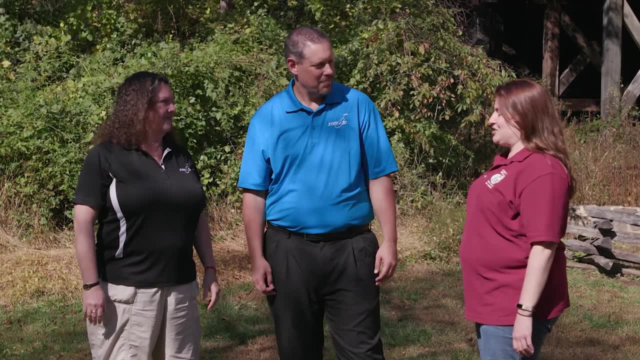 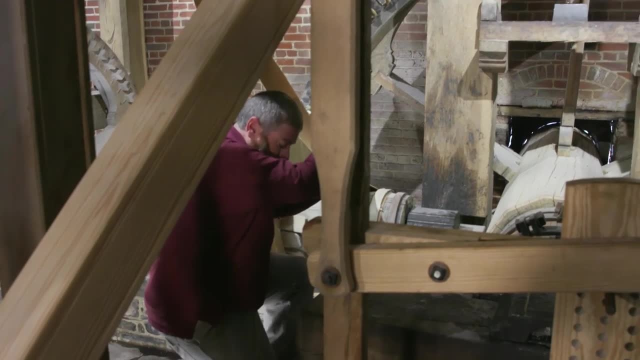 have 200 years ago, using water power and lots of simple machines. Colvin Run Mill in Great Falls, Virginia, was built circa 1811.. It is one of the few surviving operational 19th century water-powered grist mills in the Washington DC area. 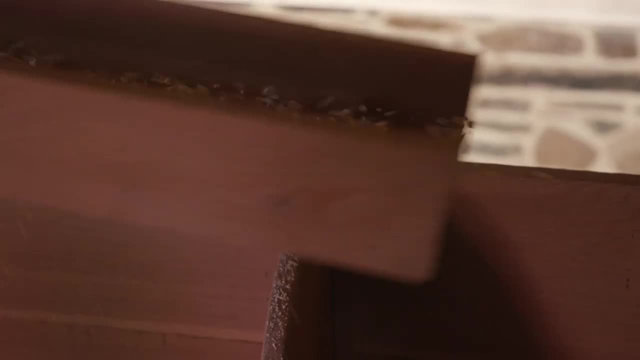 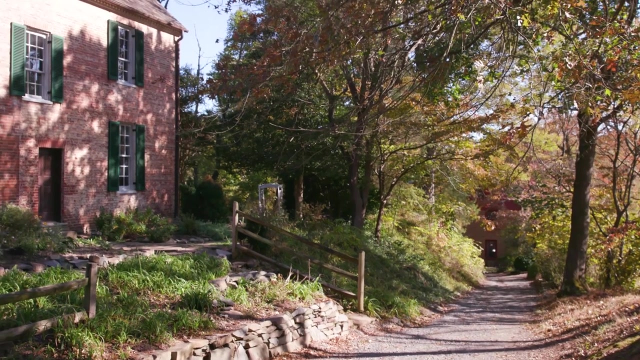 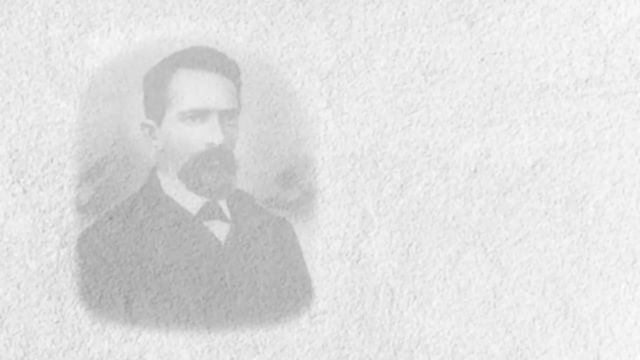 Its restored mechanism is a nationally significant example of automated technologies pioneered in milling and later adopted across American industry. Down the gravel path of the park is the miller's house, home to some of the families who owned and operated the mill. In 1883, Addison Millard moved his family here. 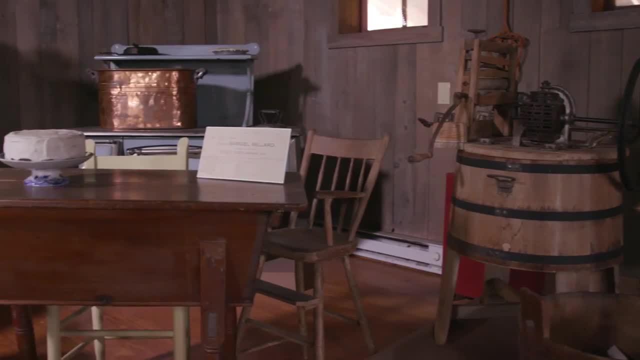 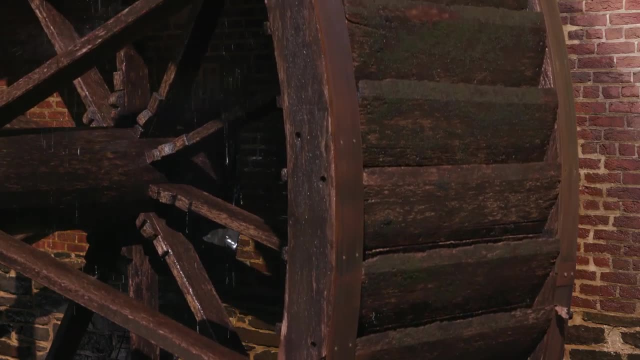 When he was 18, he moved his family here. When he bought the old mill Addison, his wife Emma and some of their 20 children lived in that house. When Addison died, the family stayed and operated the mill until 1934. 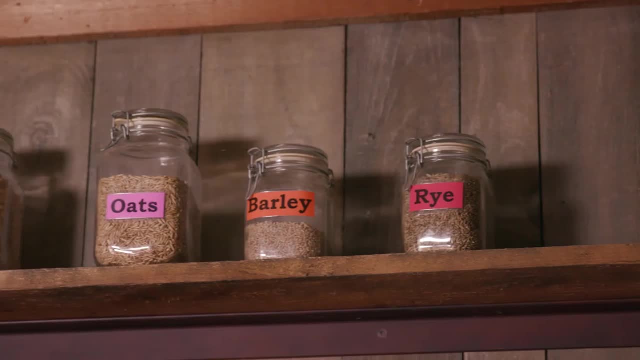 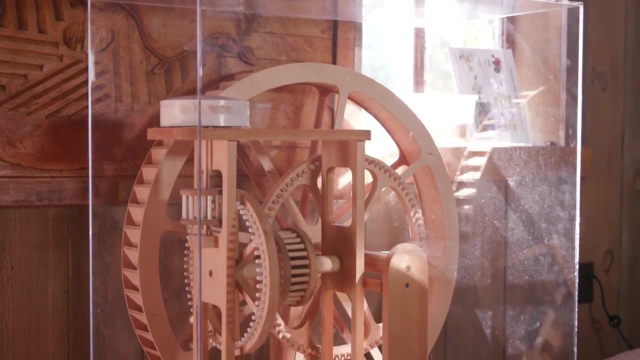 The mill was acquired by Fairfax County Park Authority, which runs it today, Open to the public. the mill runs a variety of programs for schools, scouts and the community. I've got some friends here to help us out today. Nice, Come on in guys. 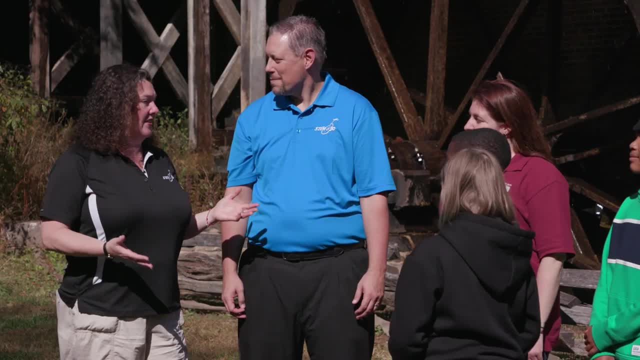 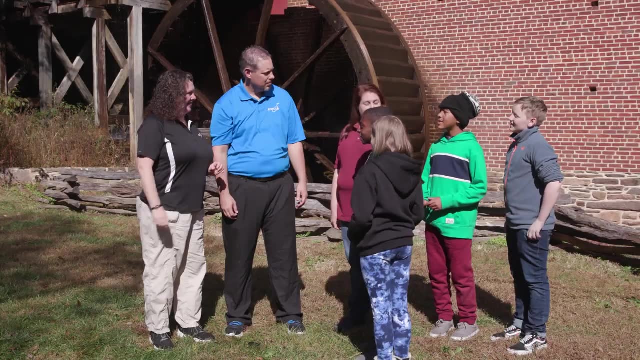 Hi everybody, Hello, Hi. Well, we're getting ready to go into the mill and we're going to be looking for simple machines. but let's take a quiz first. How many simple machines are there? Six, Six, Good job. 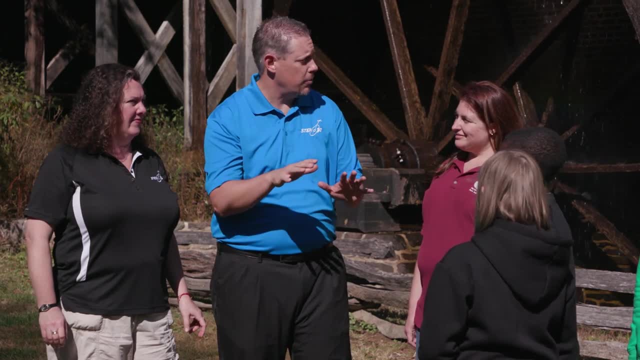 Before we head inside. just know that it's really loud in there. We're going to watch the mill for a little bit and then we'll turn it off and we'll have a little conversation. Cool, Yes, You all ready to go in? 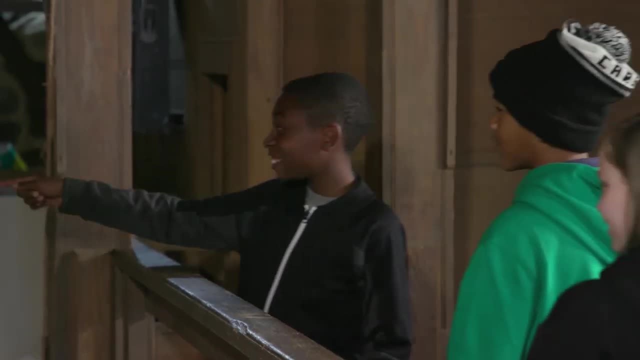 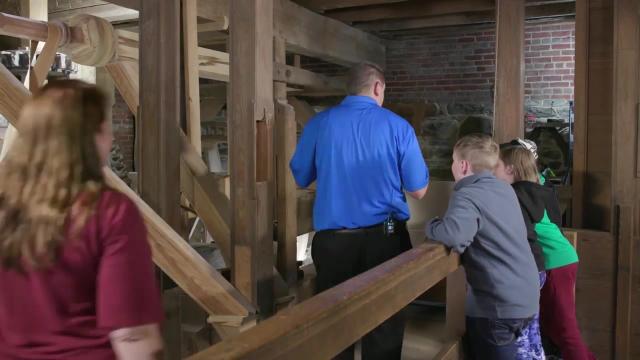 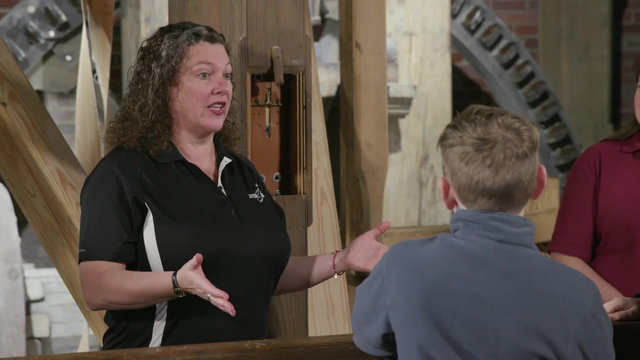 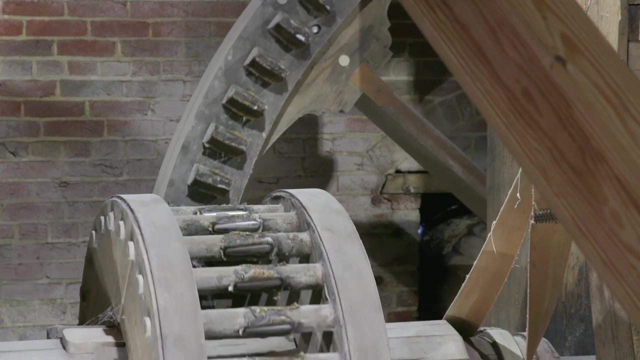 Yes, Let's go. All right, let's shut her down. What simple machine did you notice really working in here? Wheel and axle, Wheel and axle. That's right, Exactly right, Kathryn. what's going on in here? 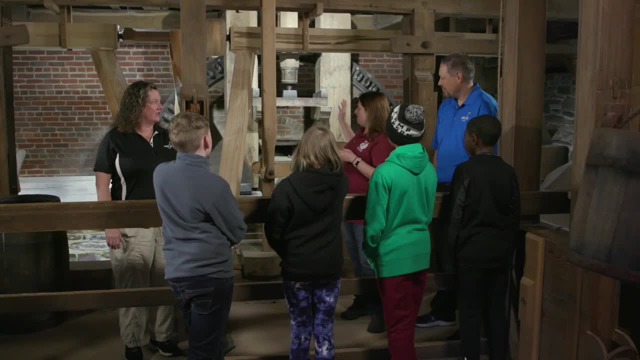 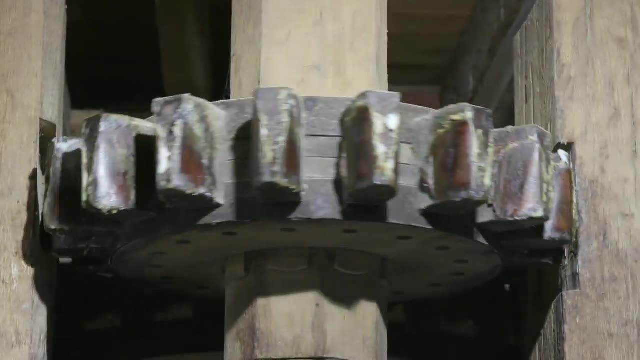 This is kind of the engine for the entire factory. All of the power is being generated here by this wheel and axle That's called the greater face gear. Gears are all wheels and axles and when we engage them, when the teeth are fitting, 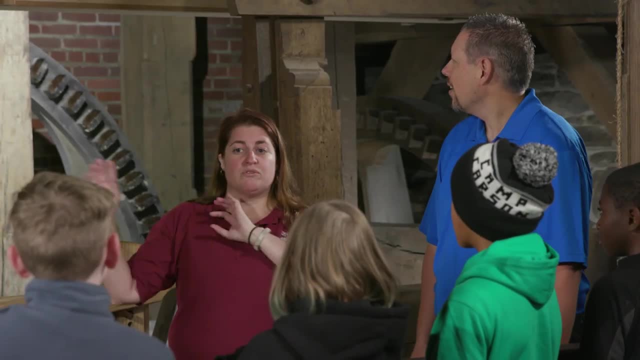 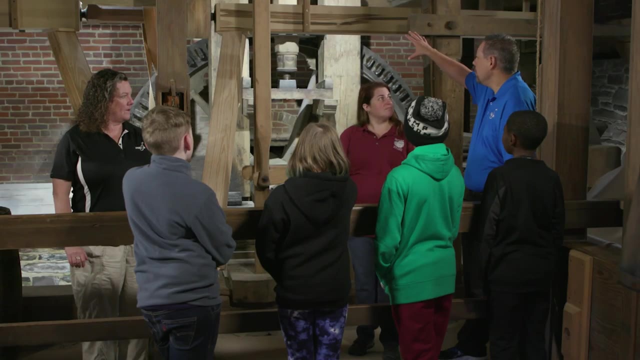 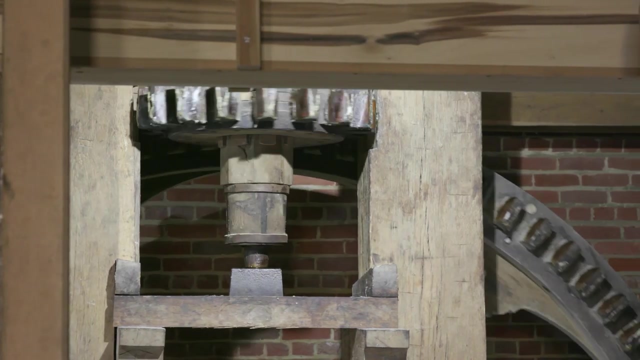 together just like a zipper. then they move one another and then we move the power to all the machines down the building and upstairs on the top three floors. Wow, And this big wheel's going around. how fast. The big wheel that you're looking at right now is going around 10 times a minute. 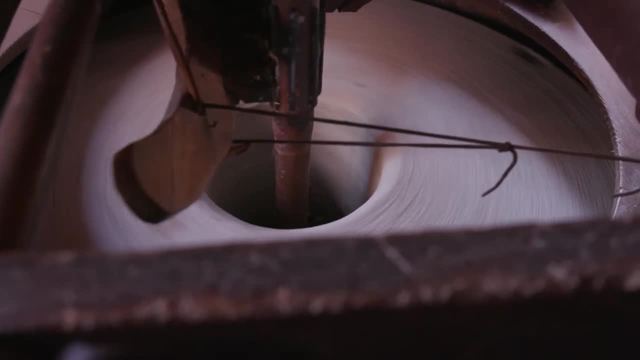 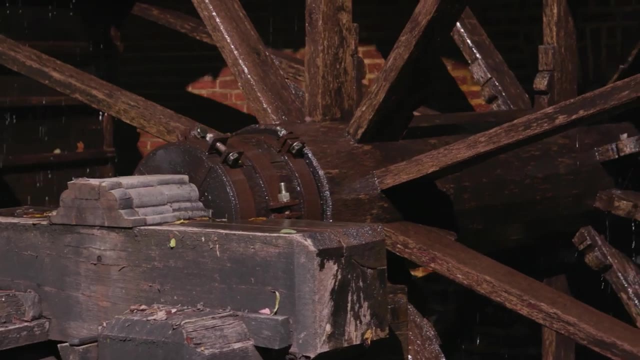 and the grindstones that we're using to create the flour is going around about 100 times a minute. Wow, Why does that happen? Well, the gears outside have to spin fast enough to power all of the other gears here in the building. 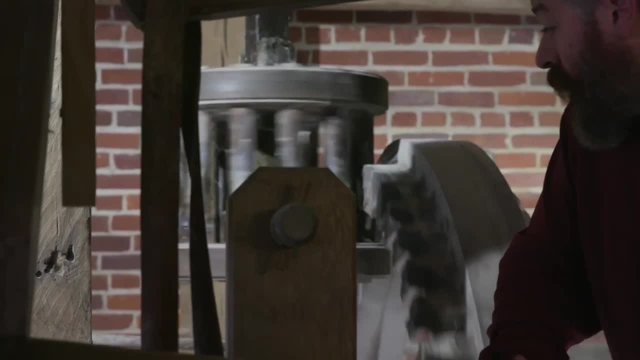 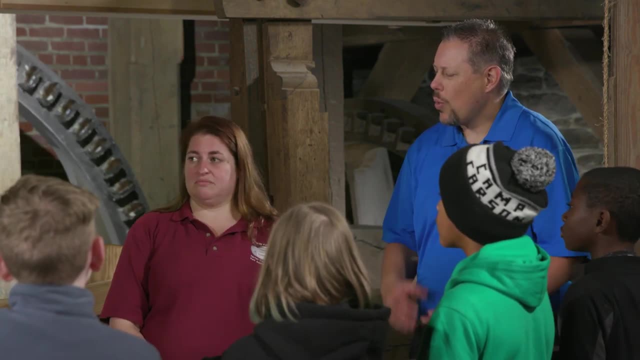 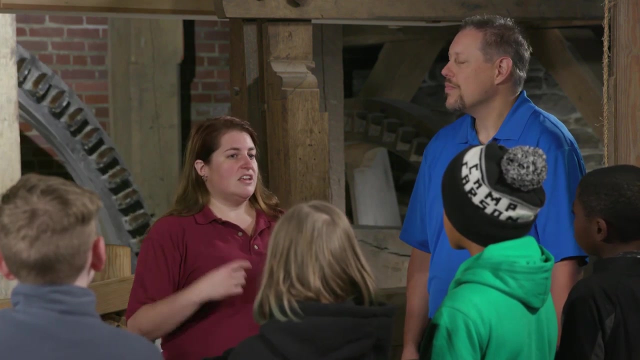 So when that's going fast enough, it makes the smaller gears go even faster. Everything in here is basically a machine, and all of those gears are what are powering the other machines. And why does it have to go so fast? It has to go so fast because we're taking the power a long distance. 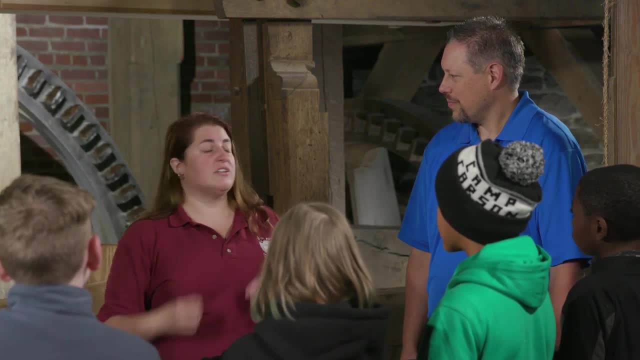 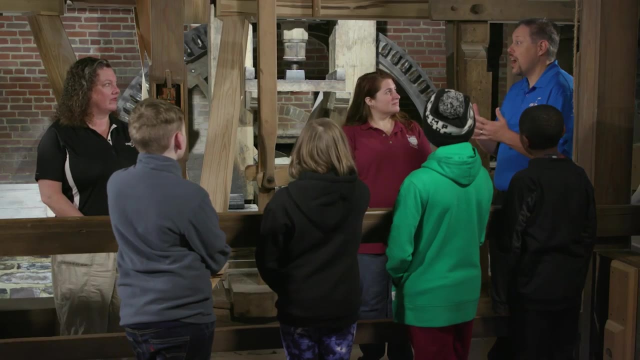 So we get it going fast enough so that when it's on the other side of the building or upstairs on the third floor, we still have enough of that power to move all of the other machinery. This reminds me a lot of a couple of other factories that we've seen. 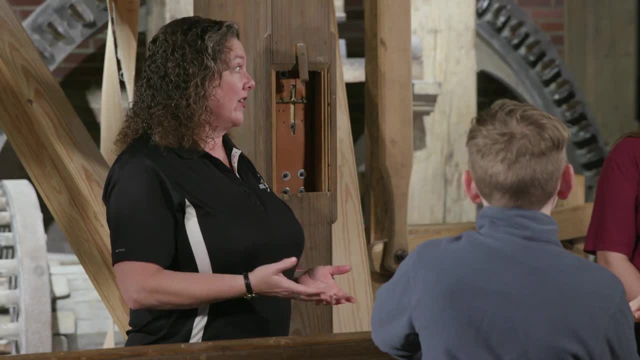 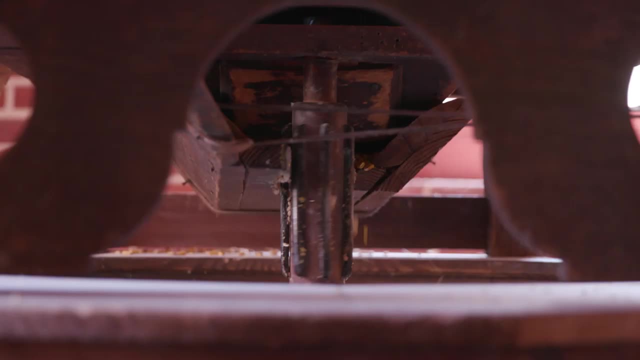 Right like the Wright Cycle Shop at the Henry Ford in Dearborn, Michigan and a very early Boeing plant that we saw at the Museum of Flight in Seattle. Colvin Run Mill is a 200-year-old mill used to grind grain and corn. 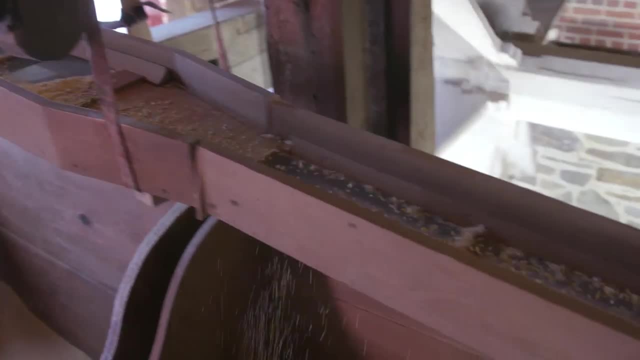 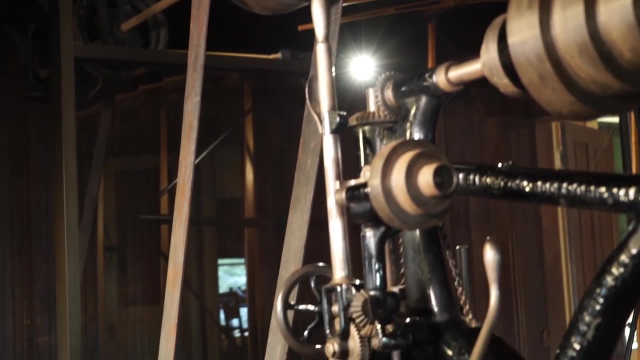 Even though they were used for different purposes. you can see similarities between the mill and the Wright Brothers Bike Shop and the first Boeing Airplane Factory. The Wright Brothers had a series of interconnected machines. Their shop had a different power source than the mill. 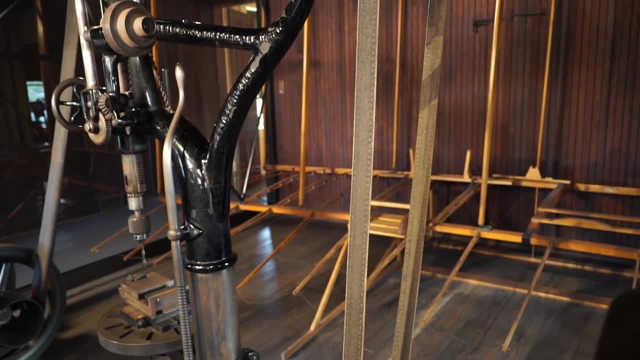 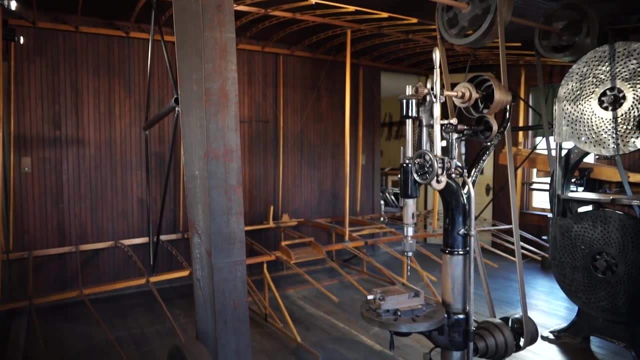 Their lathe, drill press, grinder and wind tunnel were powered off of a natural gas engine. The main problem with their shop was that it wasn't big enough to assemble the first airplane. In Seattle Washington, Boeing built their first airplane production facility. 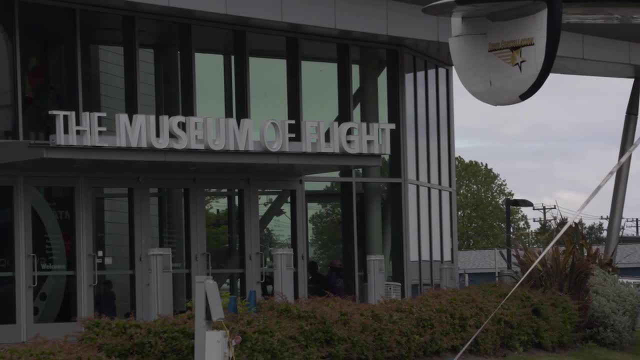 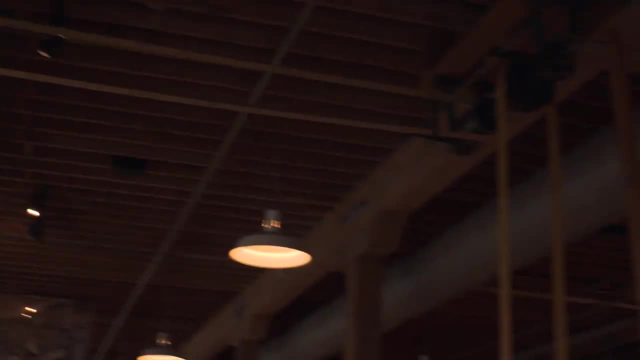 They had over 20 billion dollars. One of the buildings, one of which is now part of the Museum of Flight. Here they built components of airplanes using a series of simple and complex machines. We're in a 200-year-old mill today, but the simple machines that they used back then. 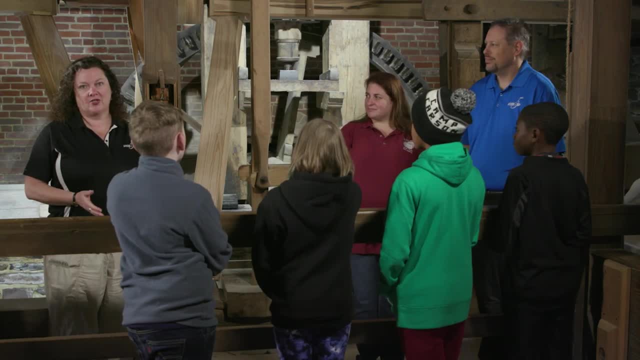 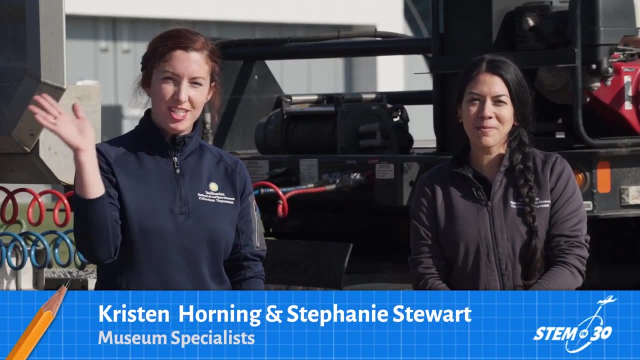 we still use today. Let's go to the National Air and Space Museum and take a look at how we use the wheel and axle there. Let's roll Hi. I'm Stephanie Stewart And I'm Kristen Horning And we are museum specialists at the National Air and Space Museum. 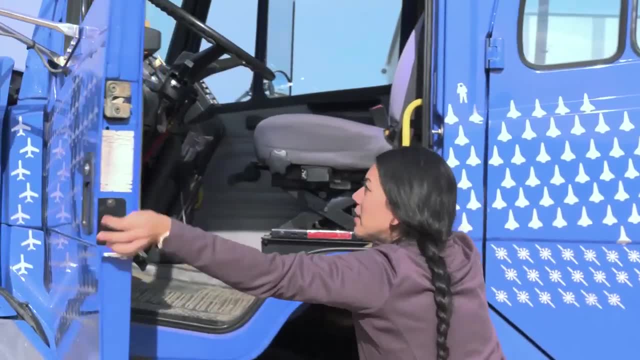 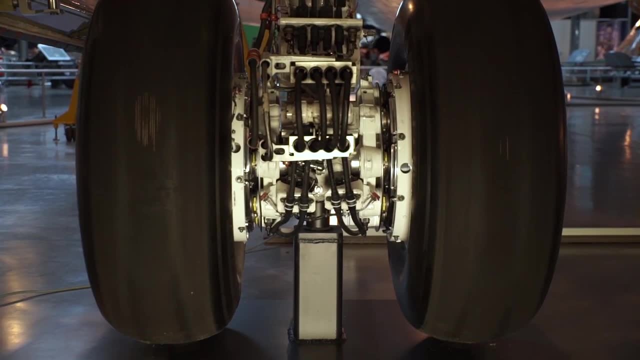 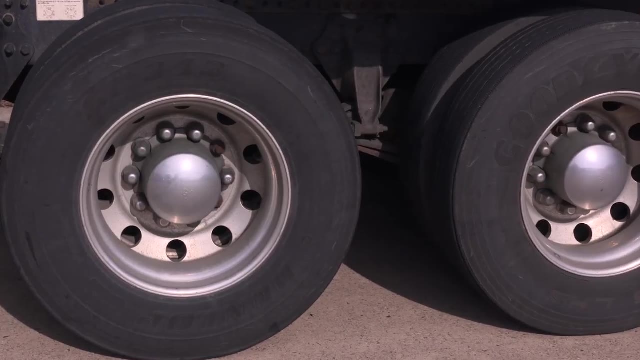 Many of the artifacts at the National Air and Space Museum use a wheel and axle. One thing you may not expect to see is a truck. It doesn't fly or go into space, but this vehicle and its use of the wheel and axle is vital to the work we do at the National Air and Space Museum. 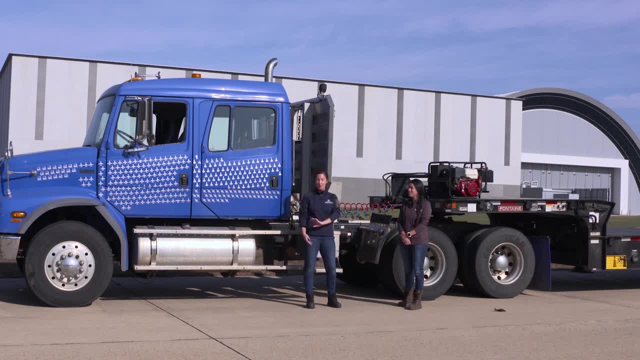 Behind us here we have our truck that we use to haul equipment. We haul artifacts between all of our museum locations So they can come out and go to the museum. They can come out to the shop, get restored and then put back on display for the public. 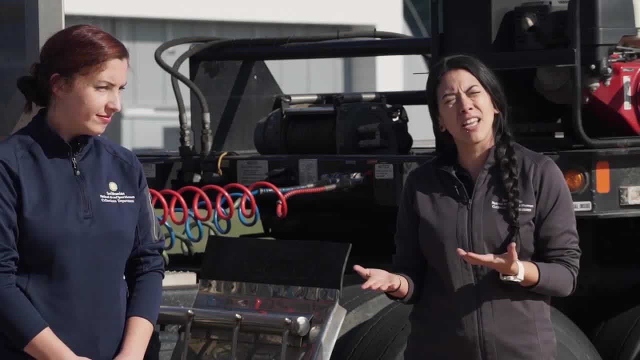 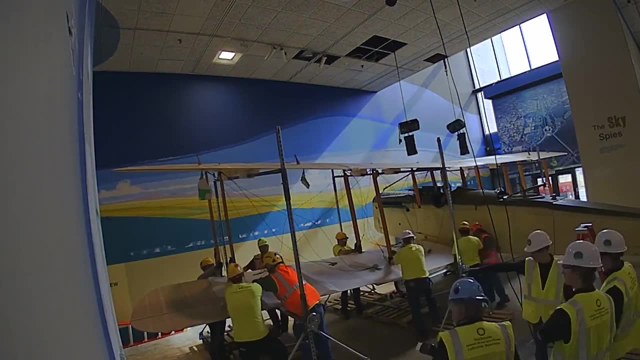 We have four different trailers that we switch between depending upon the load. So we'll have a low boy for some of our equipment, our heavier equipment, And then, if we are moving wings or fuselage, we'll be using this flatbed. 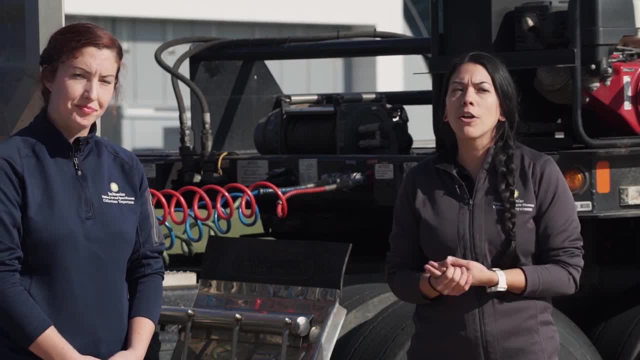 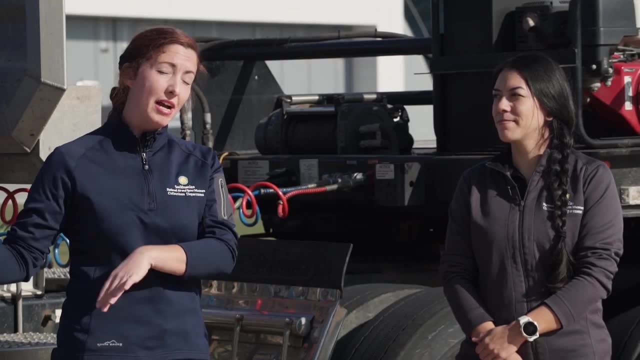 We have an enclosed trailer that we use for more delicate artifacts. Most of the time we're just doing round trips from downtown at the National Mall building site And then coming out here to Udvar-Hazy. Udvar-Hazy, We're moving out to our third facility out in Suitland, Maryland, where we keep artifacts. 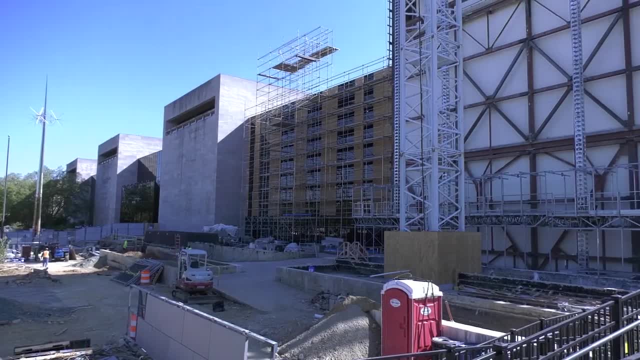 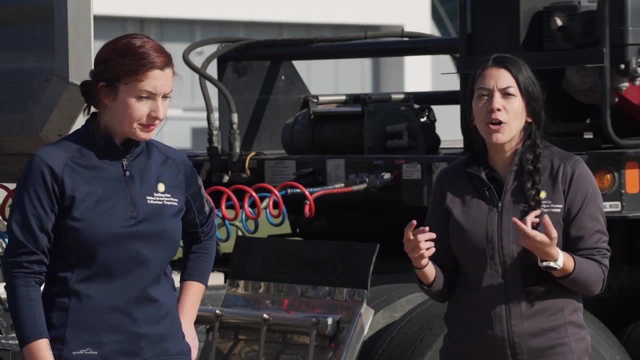 that are not on display. We have to move the artifacts from downtown to Hazy because they are renovating the building And we can't have those renovations take place while the aircraft are either suspended inside the building or just on the ground in the building because there is so much construction. 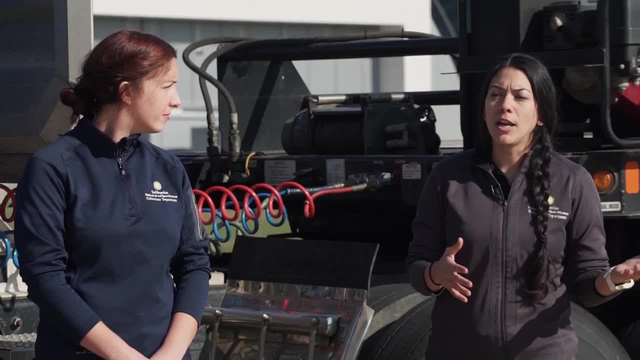 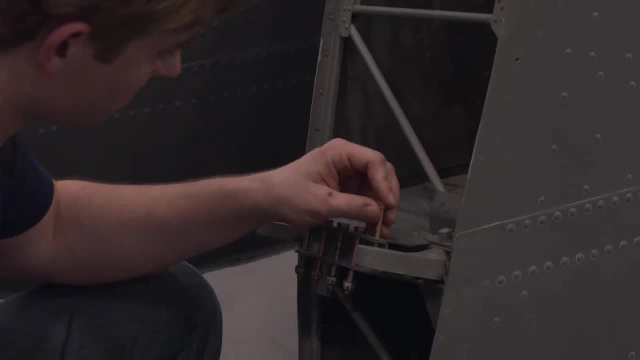 work going on around it. It would be unsafe for the artifact And we are also having the restoration and the conservation done here at the Udvar-Hazy Center, So we're able to bring it into their shop where they have the tools they need to do. 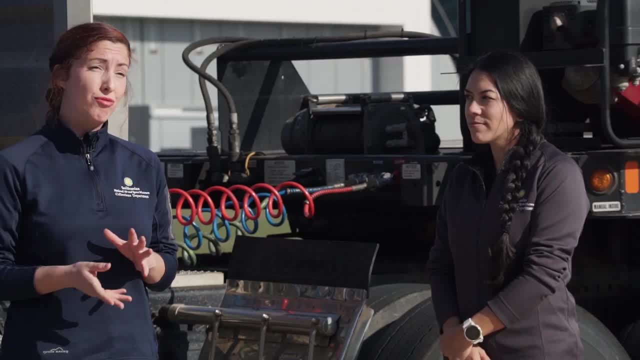 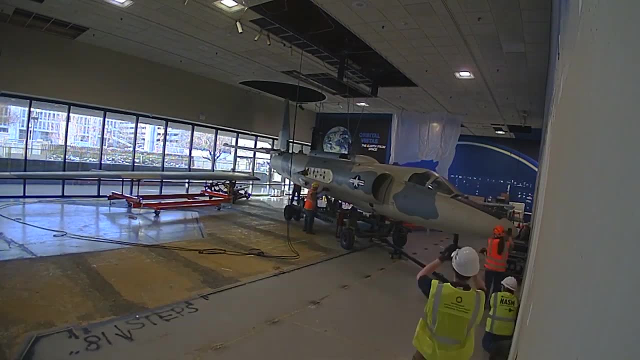 their work On any given move. we tend to have multiple teams of about four or five people that are involved at some point with disassembling- if it's an aircraft, disassembling, preparing it to get ready to move, securing it to the trailer. 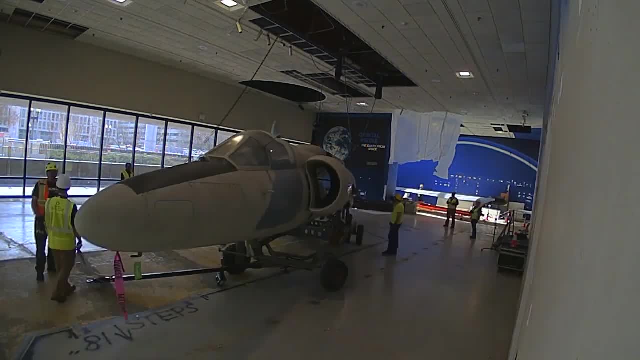 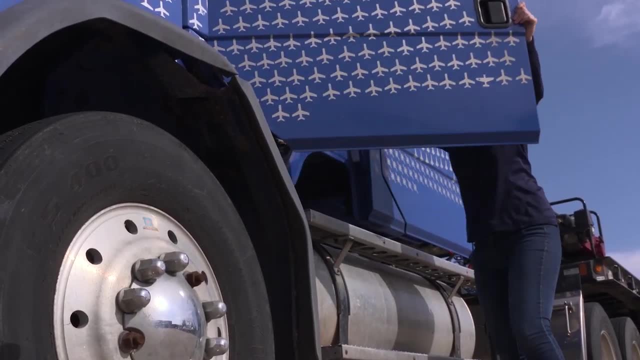 So it's quite an extensive operation. It takes quite a bit amount of people to get an aircraft apart, ready for transportation and moved to its location. You're starting to see a lot of people. Yeah, You're starting to see more and more female truck drivers out there. 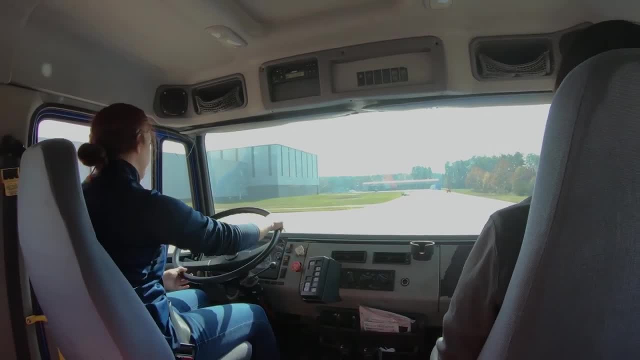 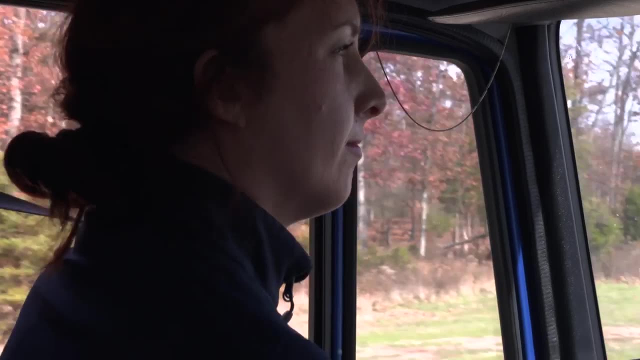 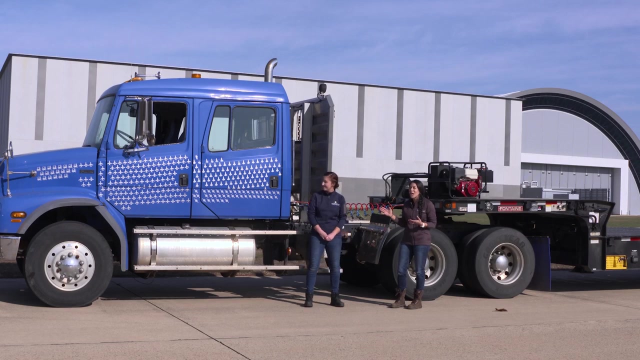 But it is pretty unusual, especially we have a staff of three right now who do have CDLs, who drive the truck, And to have two female drivers is pretty significant. You may notice we have stickers on the cab of our tractor similar to aircraft markings. 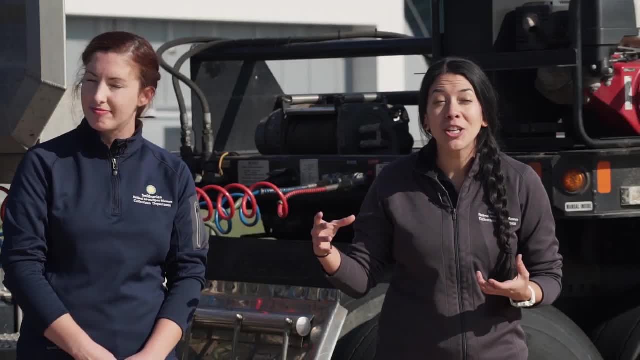 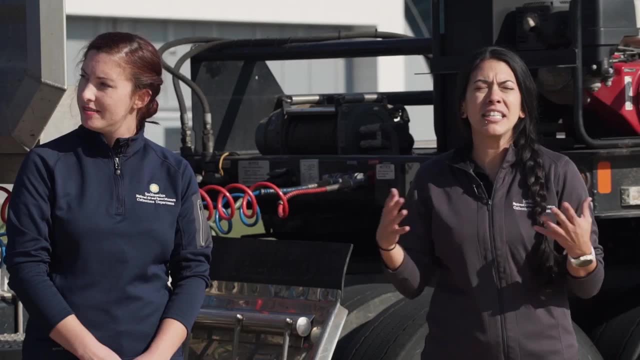 on their fuselage And many years ago, what we started to do was to place the stickers. This is a representation of different loads. You have the forklifts at the front representing the different equipment, so cranes, forklifts. 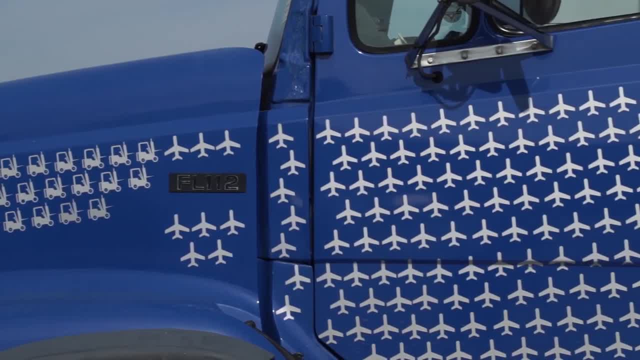 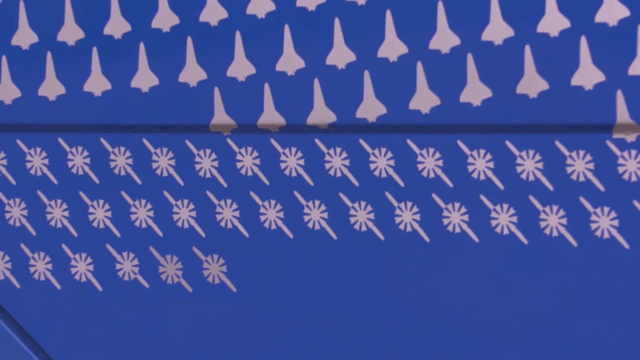 and platform lifts, And then we have the aircraft and then the shuttle to represent the different spacecraft, And then down at the bottom, radial engines, because we have moved a lot of engines over time- And then right in the center, at the very top, is a little spaceman. 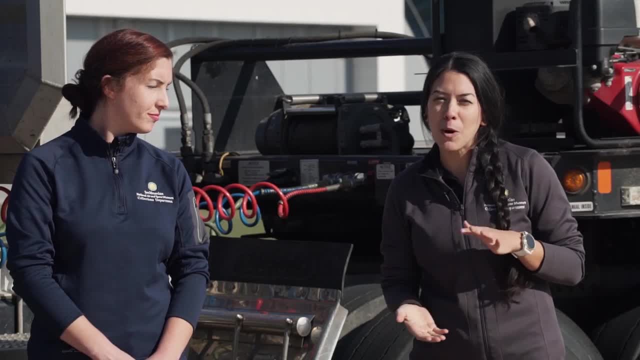 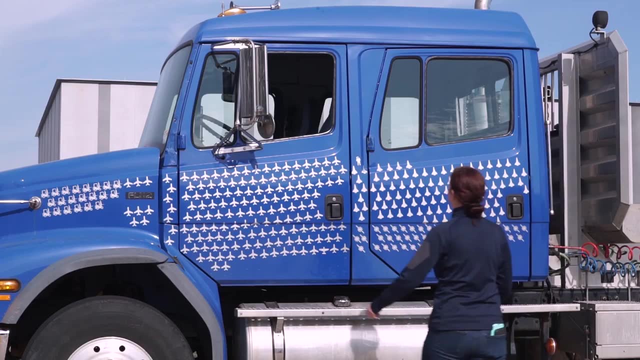 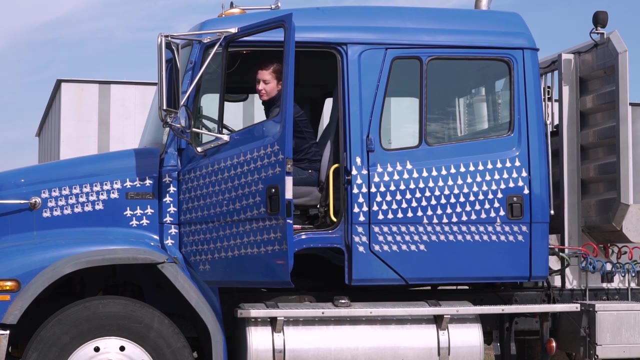 And that's to represent the many, many spacesuits that were moved over the years. This, This amount of stickers doesn't fully represent everything we've moved. We stopped putting stickers on and since then have started moving a lot more objects related to the transformation revitalization project that have not made it onto our truck yet. 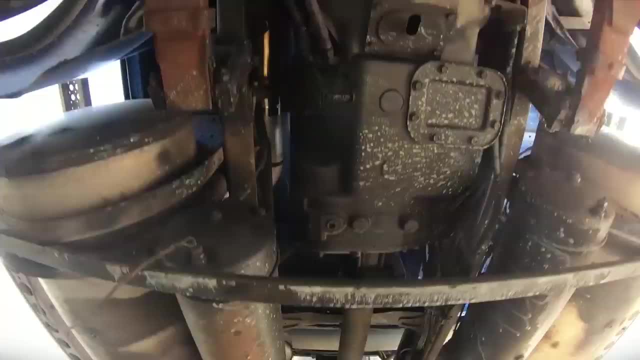 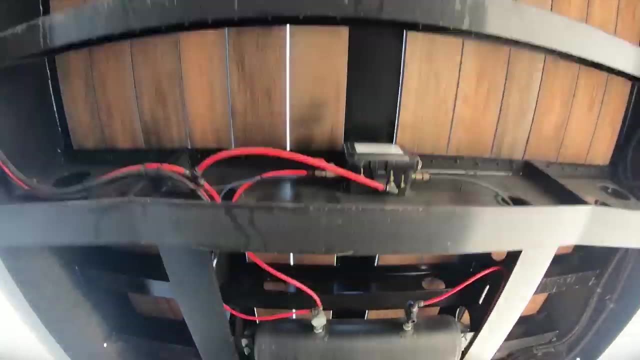 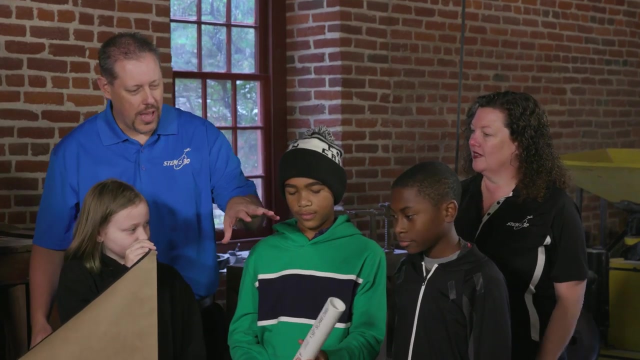 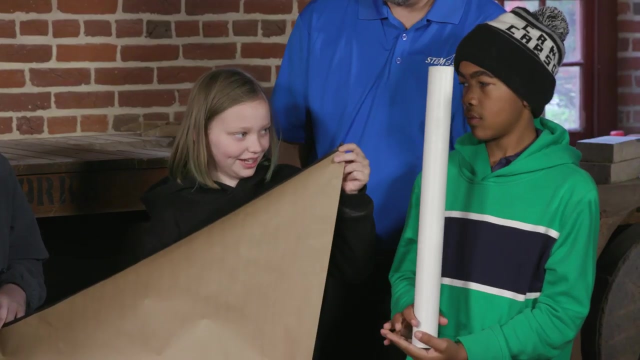 Marty, it looks like you have a simple machine demo here for us. We do So, we've got a stick here and then we have a cut out of another simple machine. What simple machine do we have here? An incline plane, That's right. 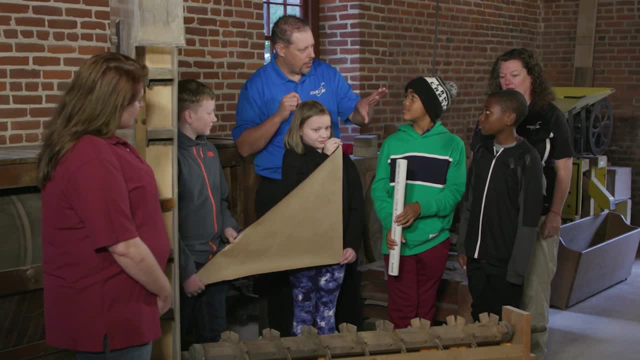 This is an incline plane, And so you guys are going to do a little demo here. We've got our tape man over on the end. Y'all are going to tape this incline plane to the stick and then we're going to wrap. 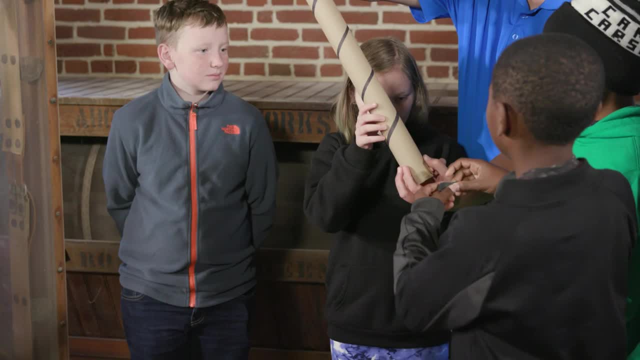 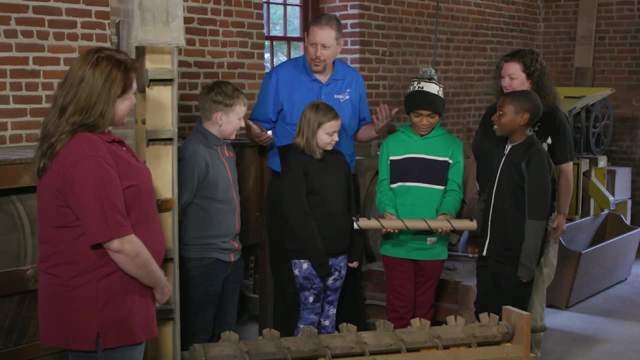 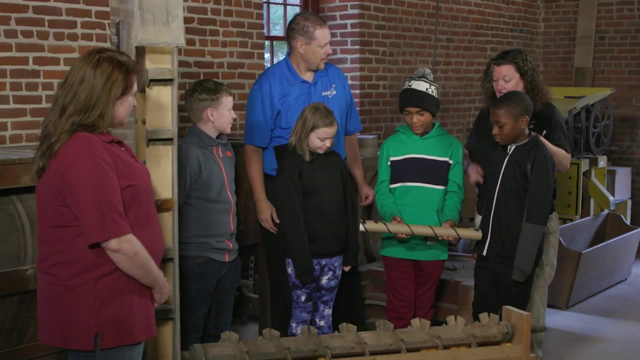 it around and see what happens. Let's tape that on the end there. Now what do we have here? It's a screw. That's exactly right. An incline plane wrapped around the stick gives us a screw. That's the only screw we're going to be looking at here. 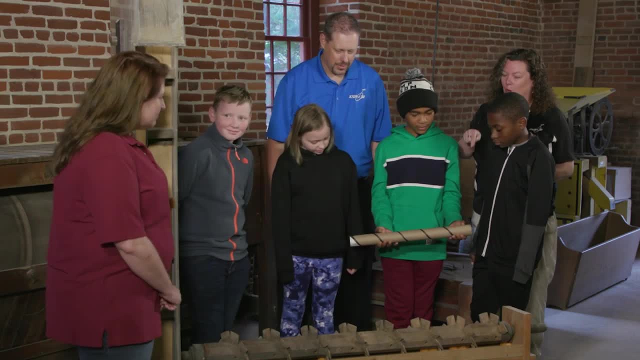 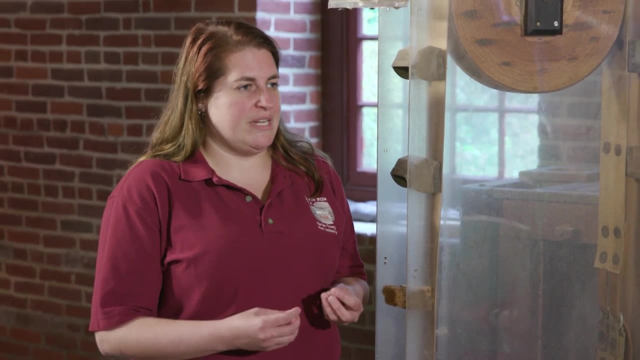 Katherine, can you tell us what is this screw and what does it do? So this is an example of an Archimedean screw, And here in our mill we use the Archimedean screw to move our grain or our flour or our cornmeal from side to side in the building. 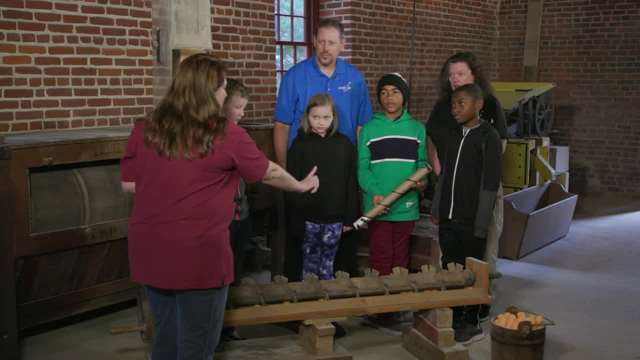 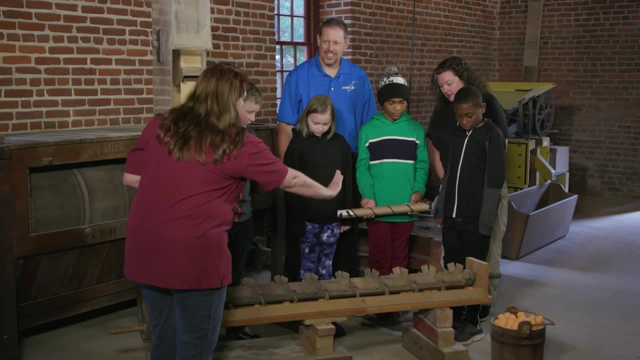 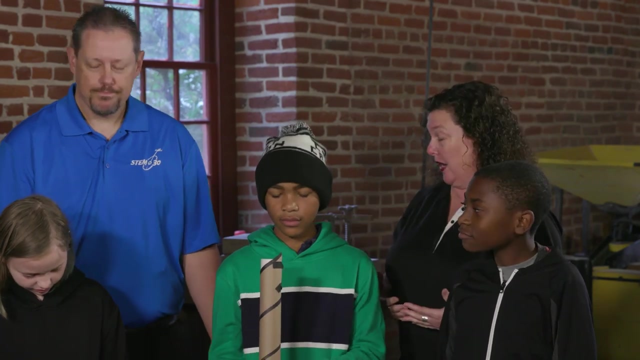 And what happens is it's poured into one end and those paddles that you see are the incline plane that are wrapped around the stick, And the paddles stay in one place but they move the grain down here to the other end. Unfortunately, we don't have any grain right now, but we do have some ping pong balls that. 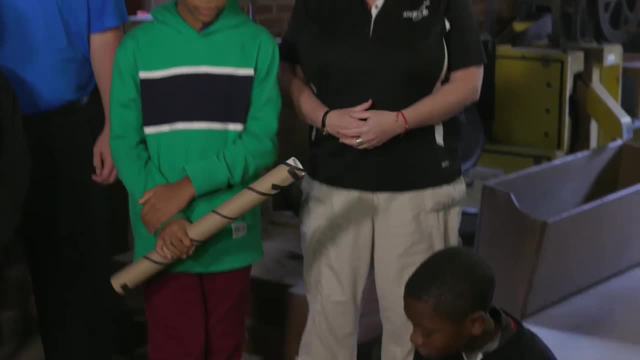 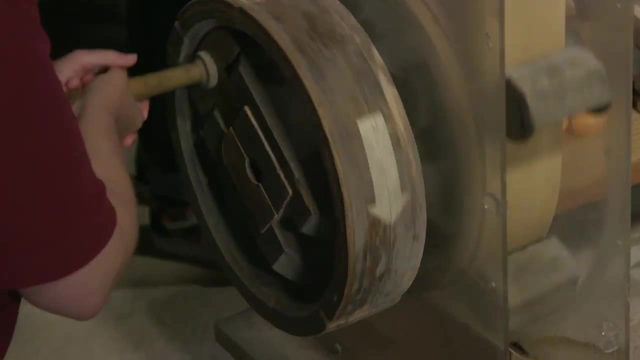 we're going to send through this. Nathaniel, why don't you load her up and let's see what happens? Let's see it in action. So the screw's going to turn and if you put our ping pong balls in, Don't get sucked into it. 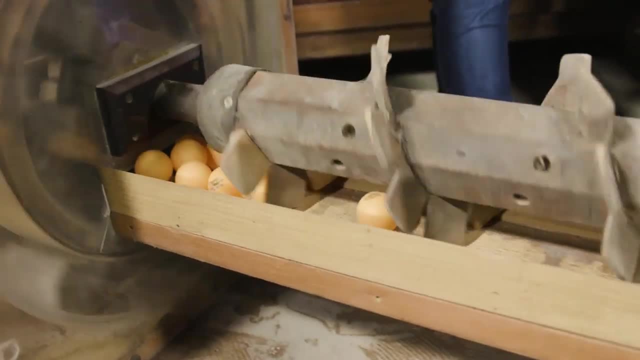 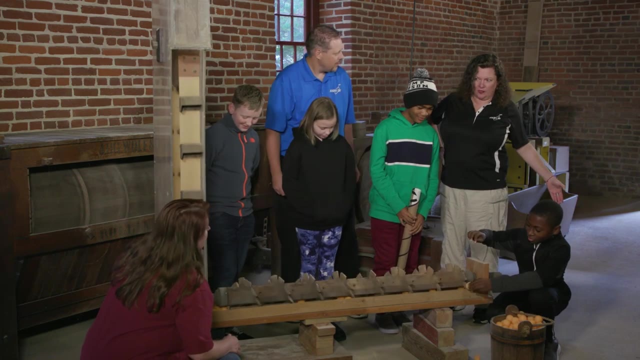 You can see how they move down here closer towards me. That is cool. You can see them that screw at work moving the ping pong balls down the stick, And this is how you move grain all the way across the mill, Move it all the way across the building. 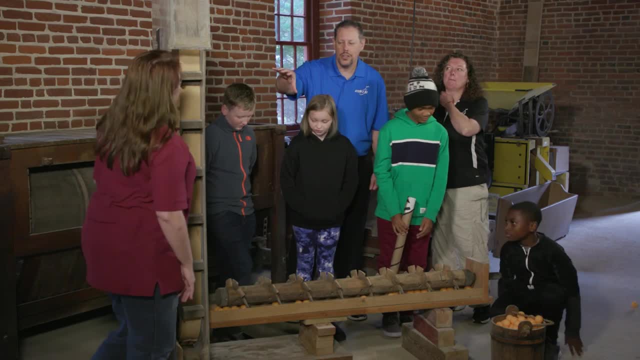 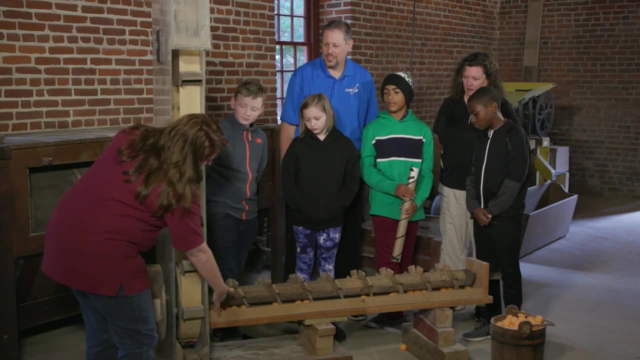 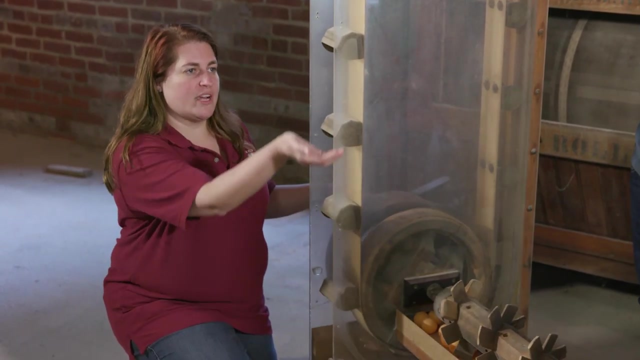 Now I see some other simple machines here at the end. What's going on there? So once we've brought the grain all the way down here to the end, it dumps it into this bottom here And our pulley- Okay, That has cups on the end- will take that scoop of grain up to a different floor. 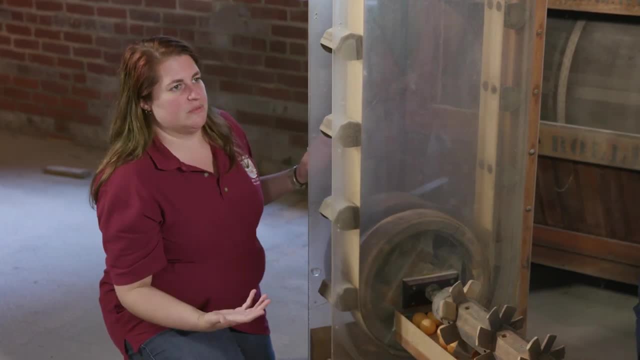 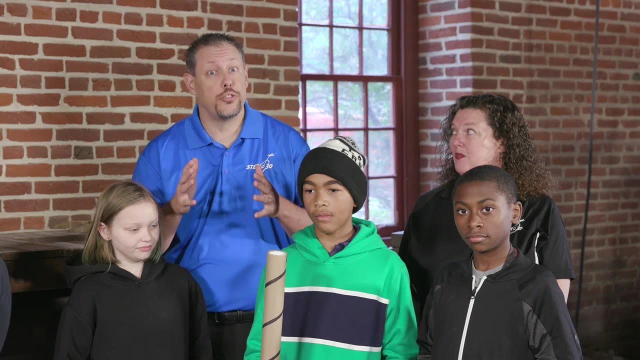 So when we move things up and down, we're using the pulley- another simple machine- so that we don't have to carry it up and down three or four flights of stairs. We use both the inclined plane and the screw at the National Air and Space Museum. but 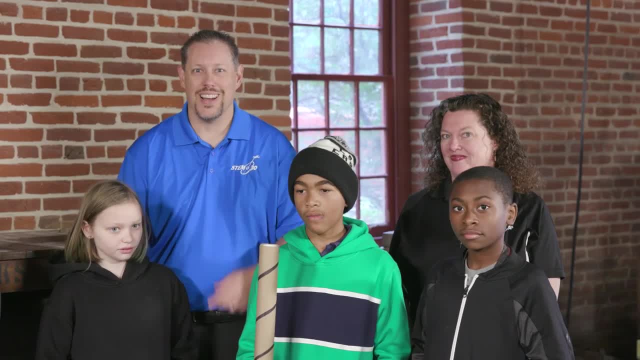 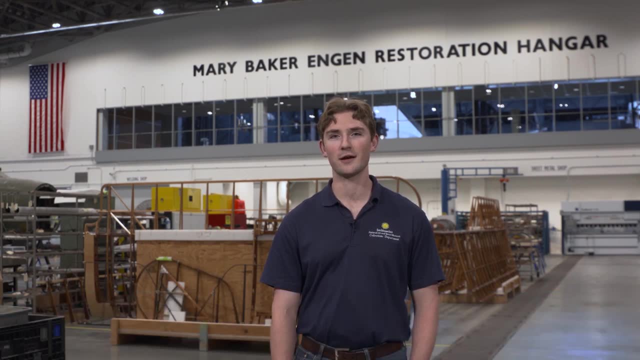 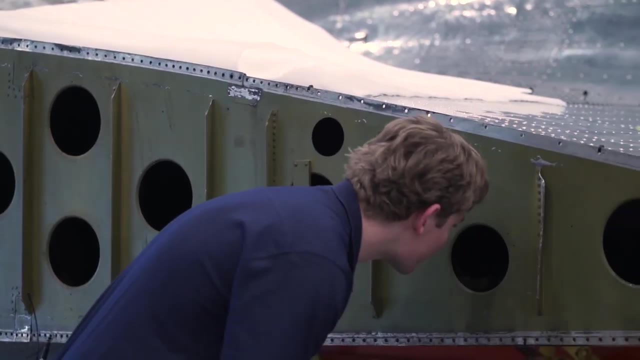 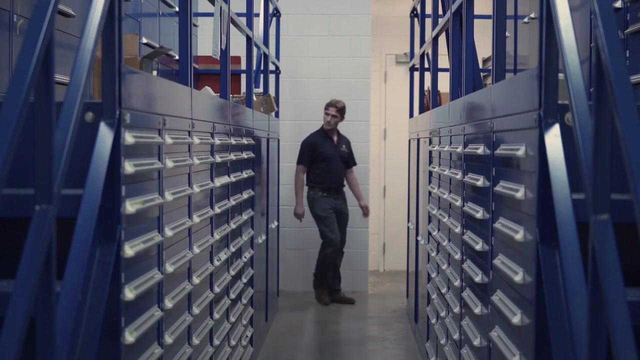 sometimes in places you might not expect. Check it out. Hi, my name is Chris Radderson. I work in the Mary Baker Engen restoration hangar here at the Stephen F Oudvaard Museum. Today we're going to be looking at some aircraft DC-3, and our tool crib, demonstrating how 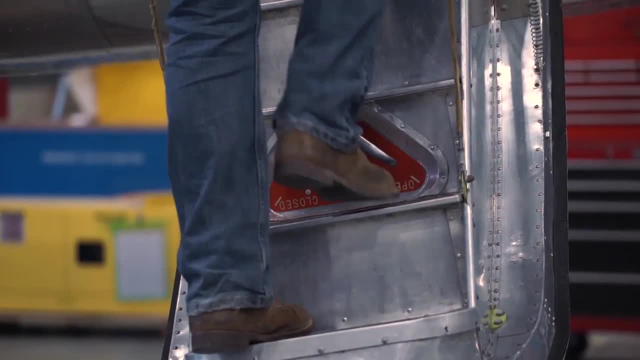 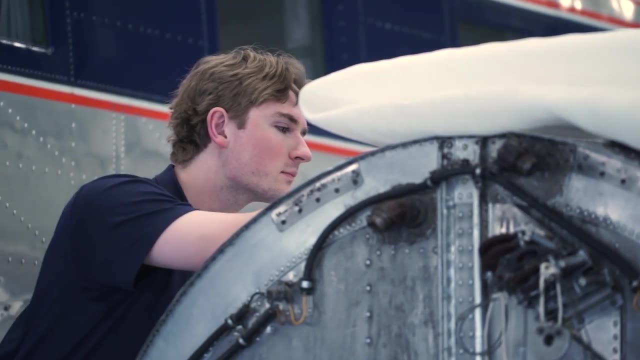 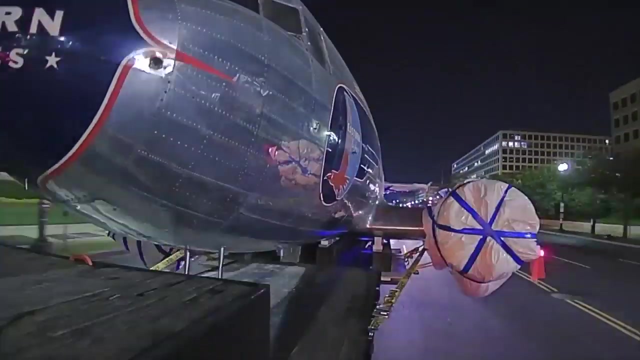 we use simple machines like screws and inclined planes in our everyday work. Here we work on some of the larger artifacts in the collection. Right now we're very busy because of a lot of the larger items from downtown having been moved out here While the museum is under construction. 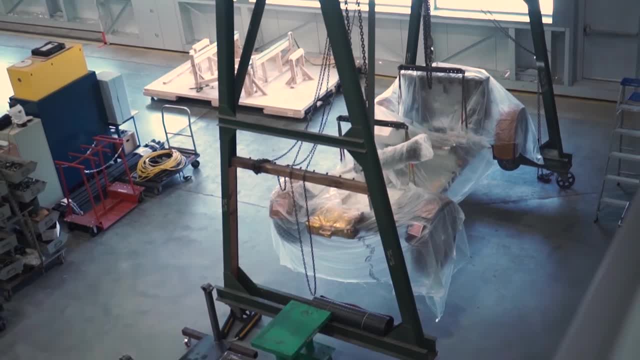 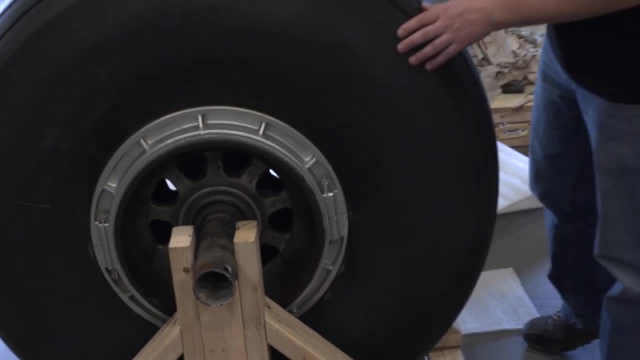 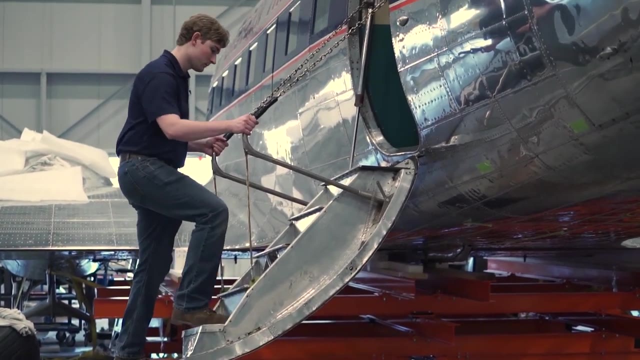 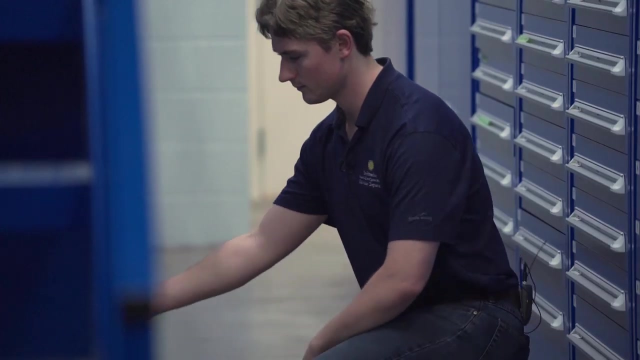 The tools we use to work on these aircraft all come back to simple machines. We use pulleys and wheels, and axles and wedges, But one that we use a lot is the inclined plane. Even though some of these are small tools or look very simple, they make a big difference. 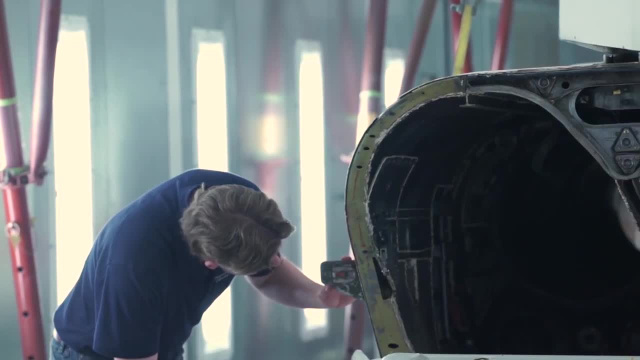 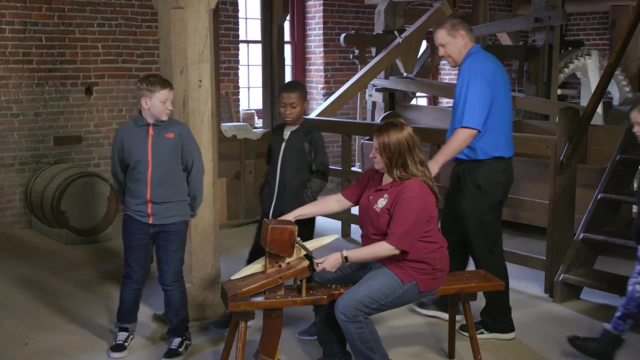 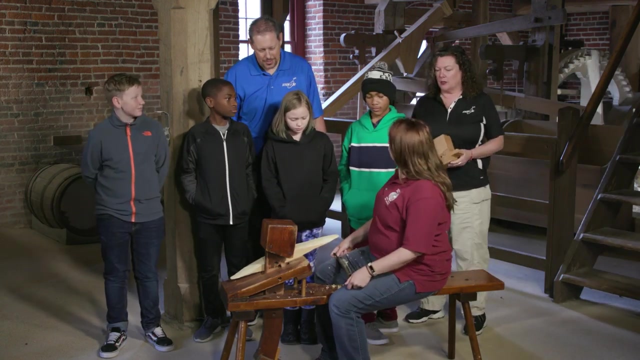 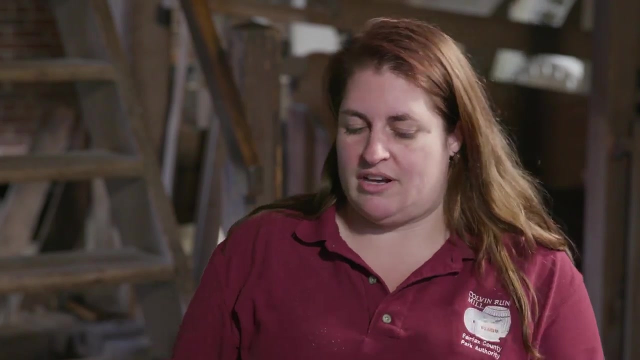 in what we are able to do when working on these priceless artifacts. Come on in. Wow, It looks like you're using another simple machine here I am, So I'm using a wedge to shape this piece of wood. So the tool that I'm using is called a draw knife, and I shave the wood so I can make useful. 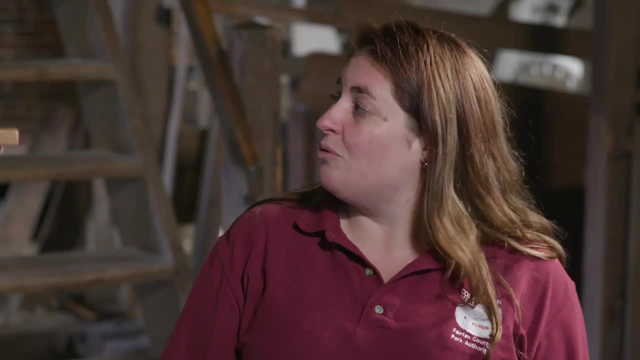 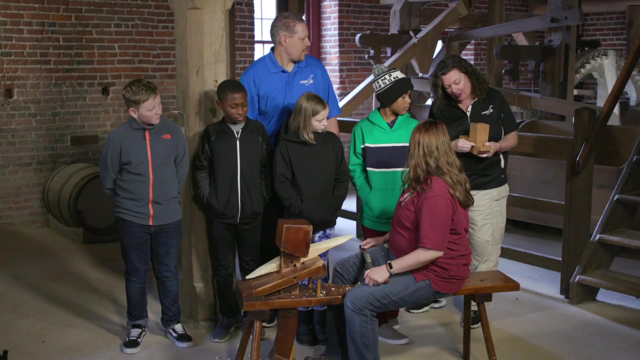 things like the legs on my shaving horse or pegs to hold this whole mill together. What do you got there, Beth? I actually have a little peg that will hold the whole mill together, So this is a model of the joint, And so I can make a round peg out of a square piece of wood. 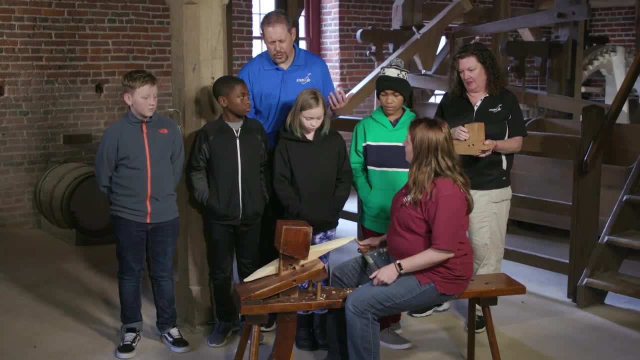 Just by shaping the piece of wood? Wouldn't it be quicker to just go to the store and buy the peg? Well, 200 years ago we couldn't just hop in our car and go to the store, We had to make them. 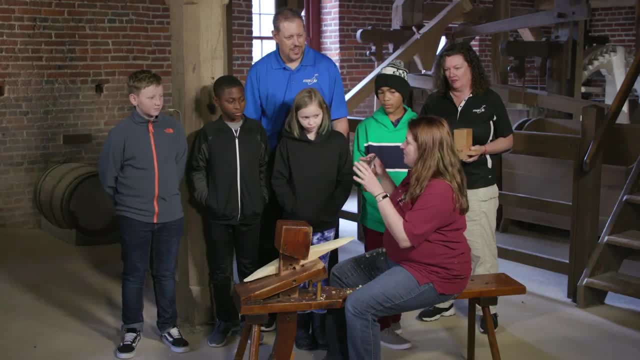 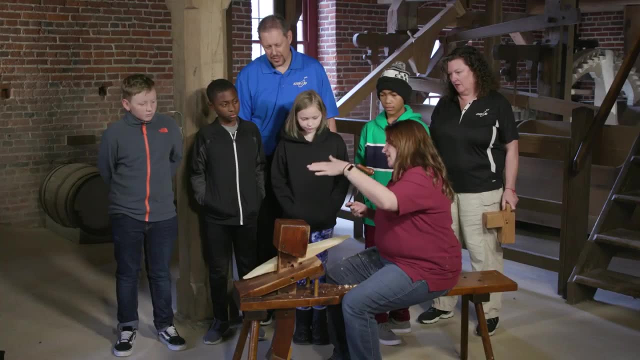 This looks like it's more than one simple machine, though It is. So our draw knife is two. We have handles, which are levers, And then the blade here, which is a wedge, And on my shaving horse, here, this is the head. 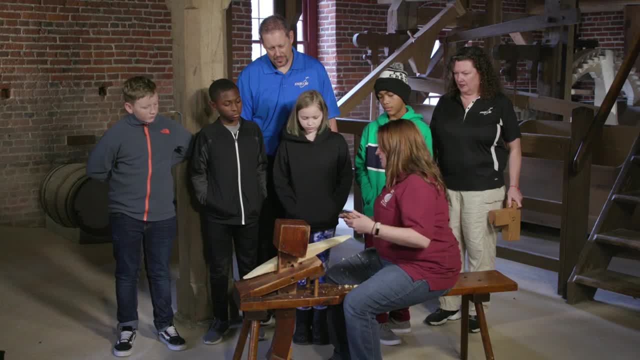 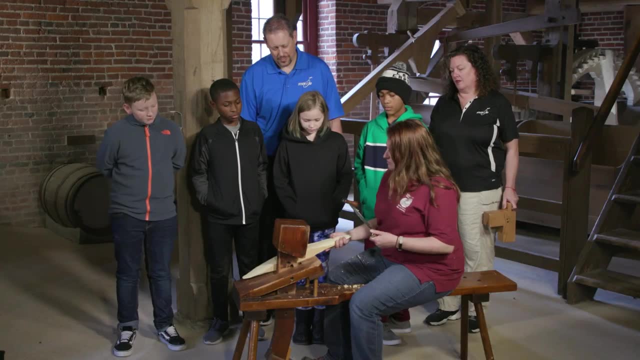 And the jaw is what's holding it in place, so it's not moving. when I'm shaving, You can see there's a fulcrum here And this whole piece here- Okay, And this whole piece- is another lever. So when I put my foot on the lever, it keeps the wood in place. 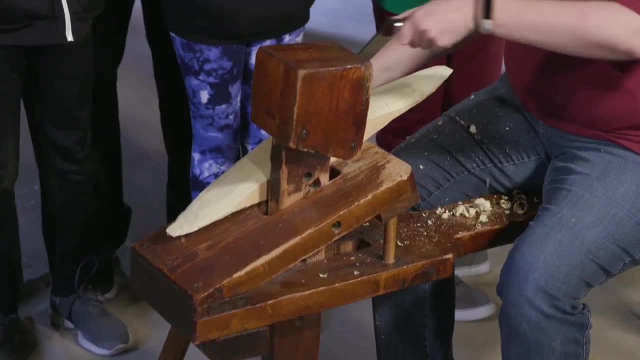 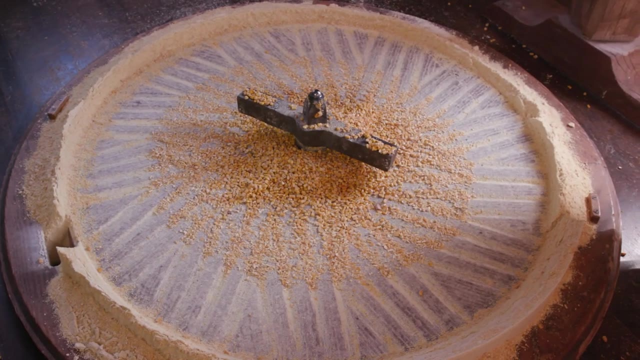 And I can use my draw knife to shape the wood. Is that the only wedge here? It's not. We actually use wedges to cut our grain really finely when we're grinding. When you have a group of simple machines working together, what do you call that? 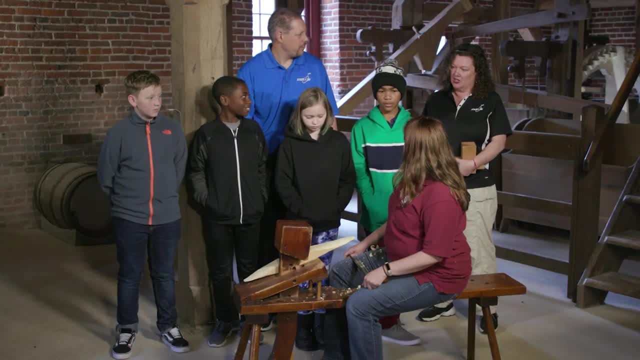 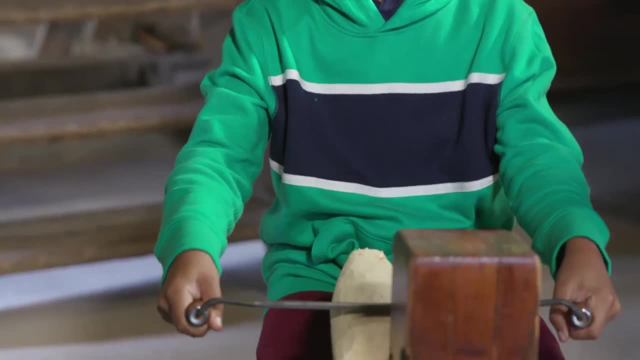 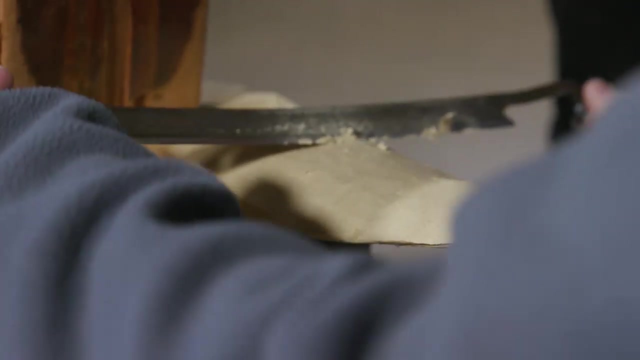 I call that a complex machine. You guys want to try the complex machine here? All right, So there's your structure. This is where I made a pile of wood. You guys can just make blocks of wood whatever they grow in the space. 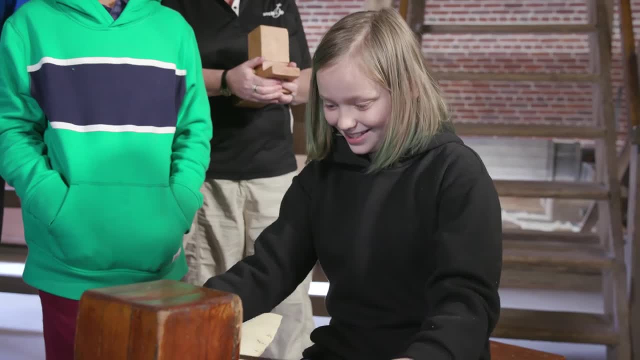 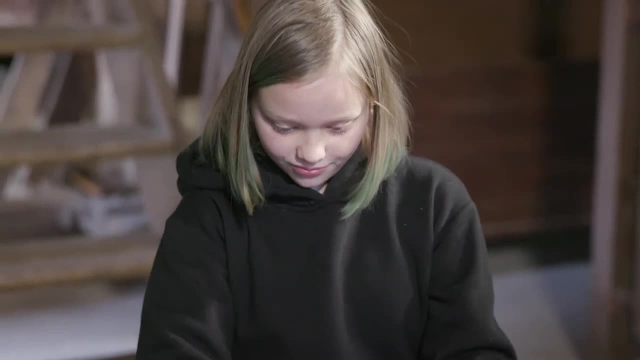 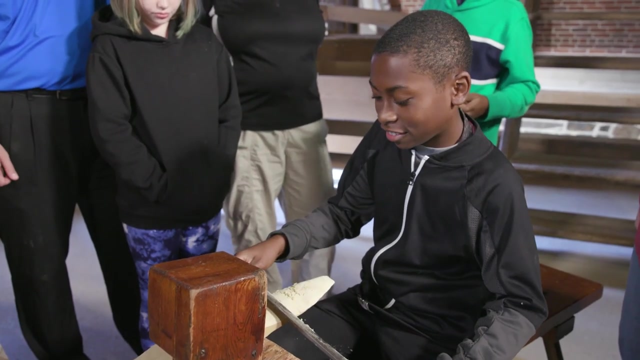 And that's that for today. I hope you guys have found this a little something interesting, If you guys like what I brought you. I hope you have a great day inse sweden. Bye. You all have done a great job using the wedge today, but do you know what my favorite kind? 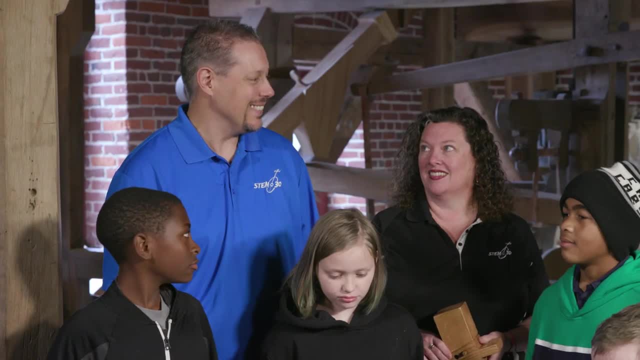 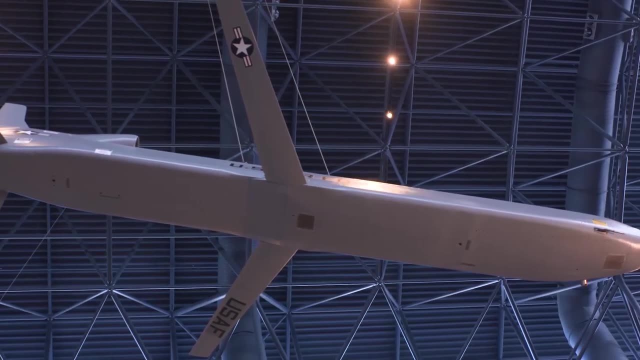 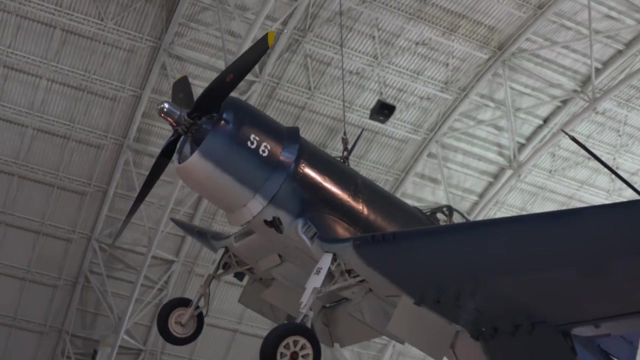 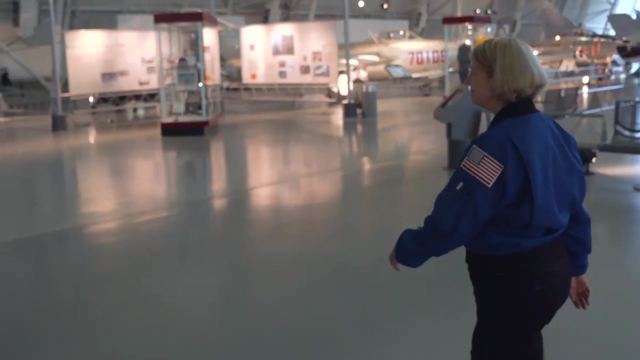 of wedge is A turkey sand wedge. Let's take a look at how we use wedges today. As you walk around the National Air and Space Museum, you get a chance to see many spectacular aircraft and spacecraft up close. However, one thing you may not notice are the simple machines that are in plain sight. 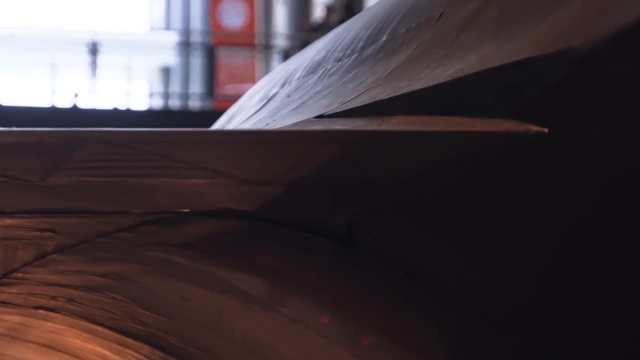 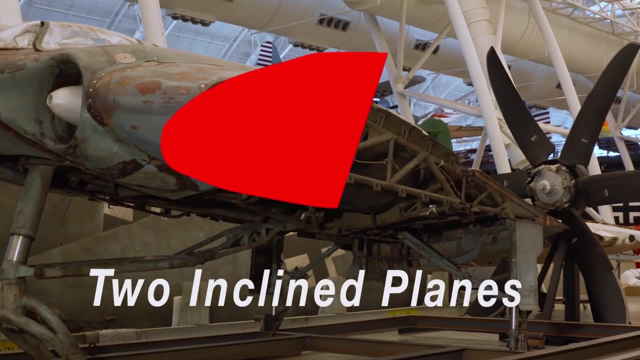 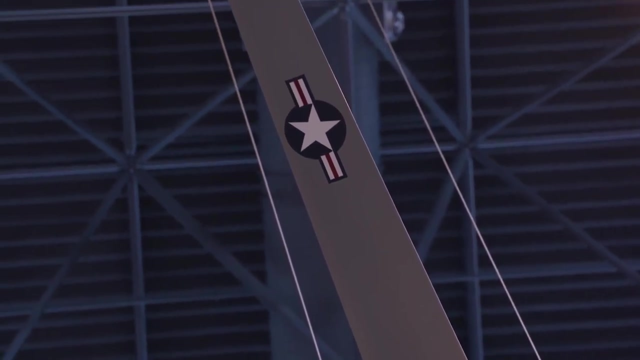 The wedge is a simple machine and a variation of the inclined plane. It has two inclined planes set back to back. The wedge is very aerodynamic. Instead of cutting through a solid, it can cut through the air and lower the resistance made by the air itself. 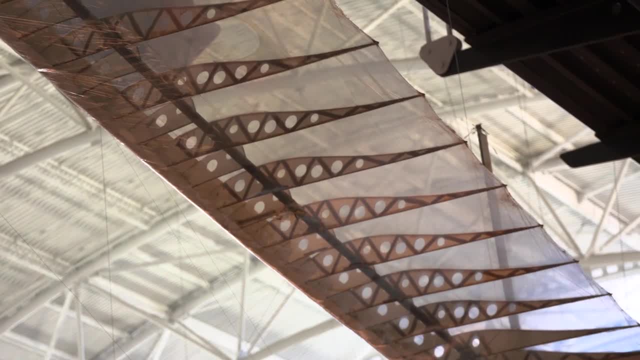 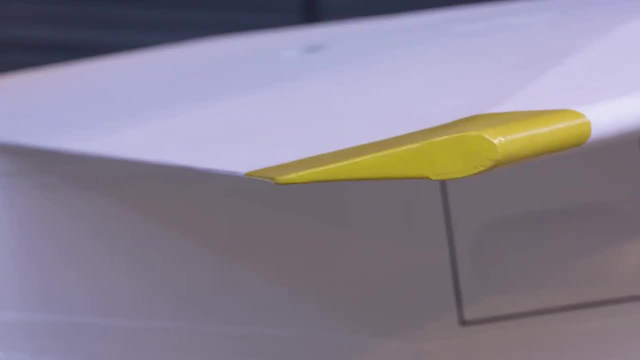 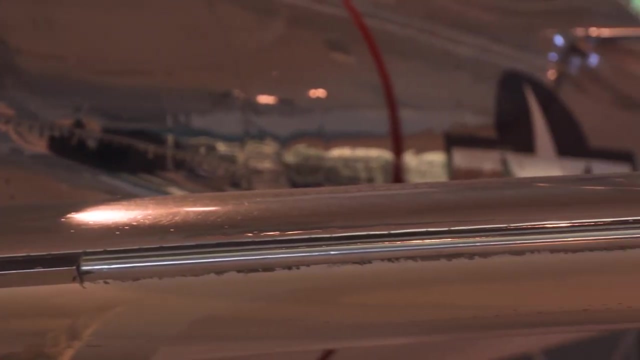 Here at the museum, once you know what you're looking for, you can see examples of wedges everywhere, From the shape of the front of airplanes and missiles to the leading edges of wings. The wings on a jet are wedges called airfoils. 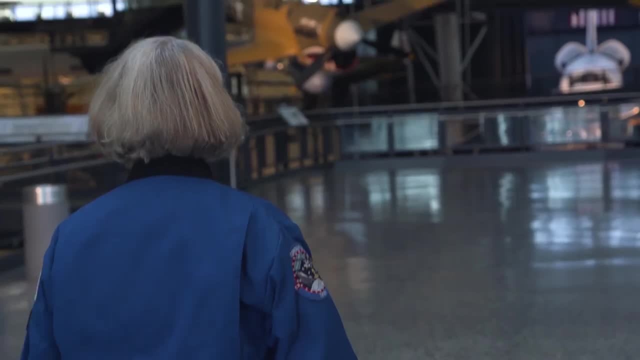 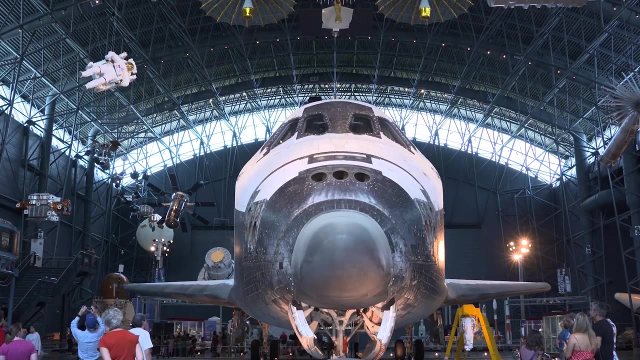 This shape allows the wings to cut through the air. The next time you visit an aviation museum or take a flight, be on the lookout for wedges hidden in plain sight. We've moved upstairs and, Claire, I have a little job for you. 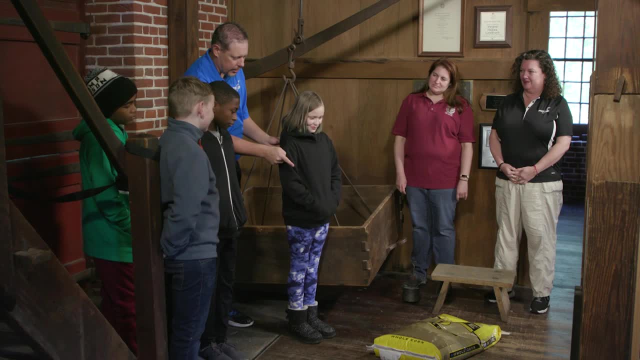 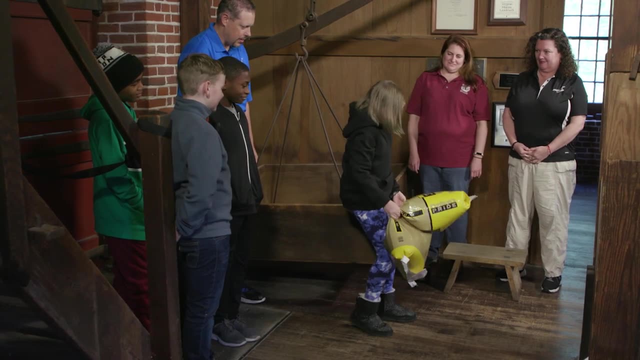 Can you help me out? We've got this bag of corn laying down here on the ground. I need you to pick that up for us. Go for it. Go ahead and set it down. That's a little on the heavy side, isn't it? 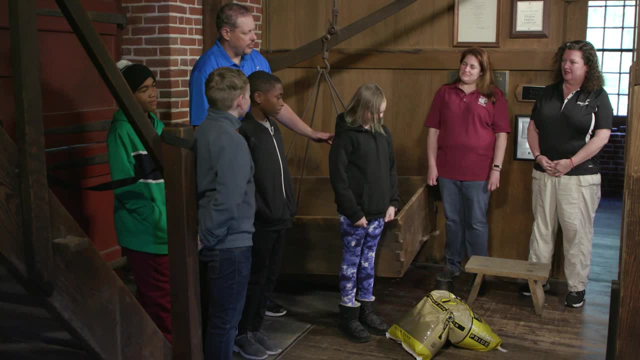 Did you struggle with that a little bit? All right, So should we make it a little bit easier, All right? Well, we've got a simple machine that can help with that. Katherine, do you want to tell us what we're looking at here? 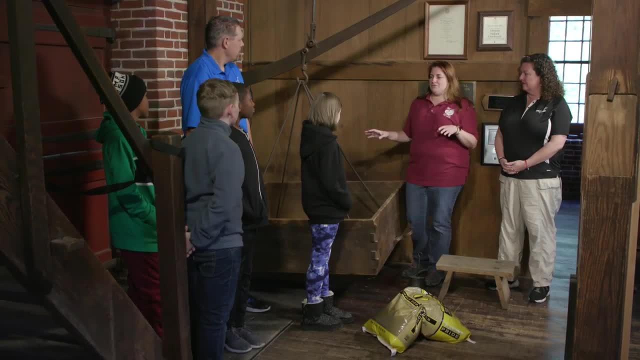 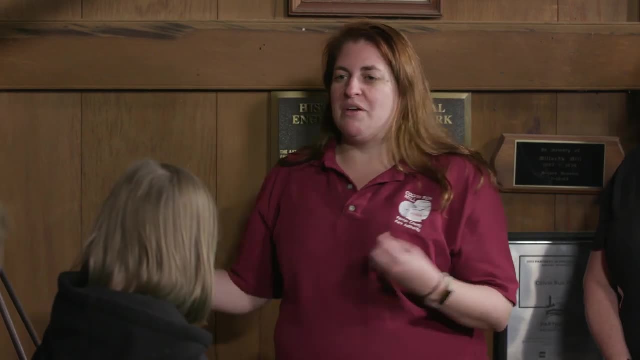 So this is what we call a beam scale, And what we would use this for is to weigh the corn that the farmers are bringing to the miller. So we wouldn't dump a bag in here. They would actually bring a wagon load of corn or a wagon load of wheat from their farms. 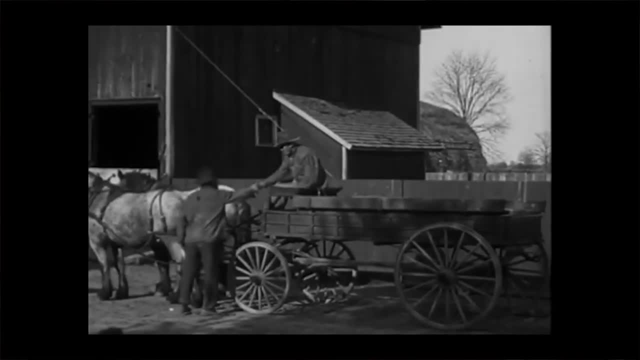 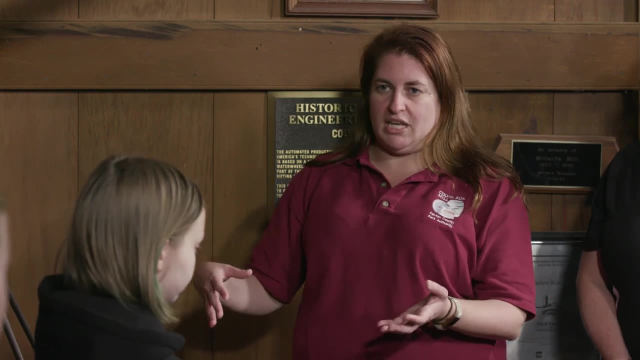 And we would weigh it here, because they would actually just sell it to the miller. So the merchant miller- this is his entire job- is taking that raw material and making a product. He doesn't have time to grow it, So the farmers bring it in, put it in the scale. 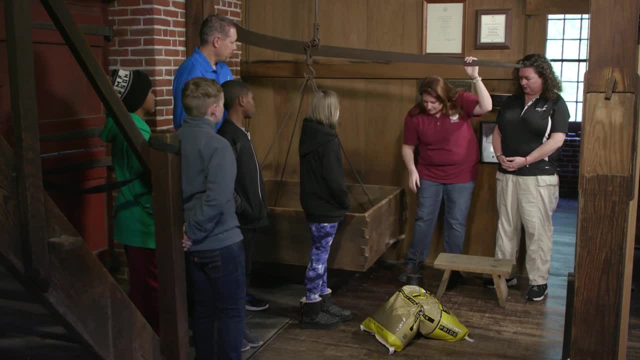 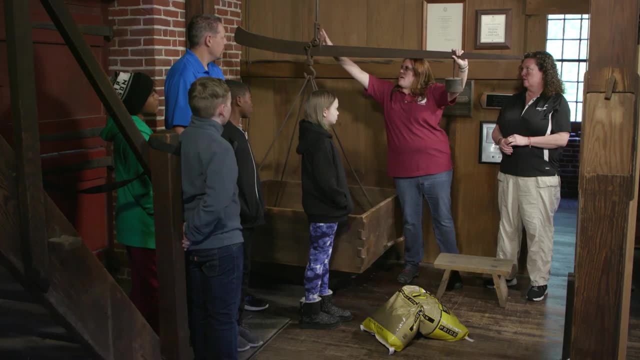 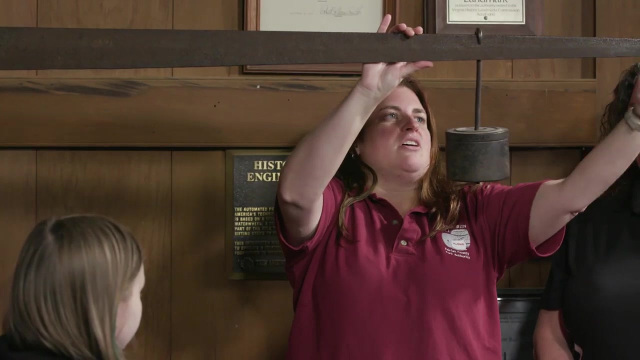 The miller can then weigh it, And what he needs is this counterweight. We put it on the beam here, this lever, And when it balances, when this fulcrum is straight up and down this point, where the lever moves, then I see where, on the arm, our counterweight is. 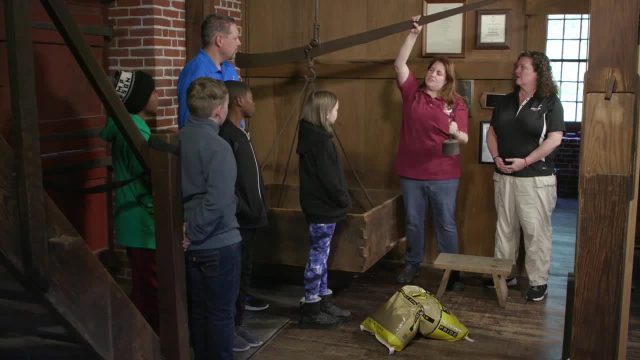 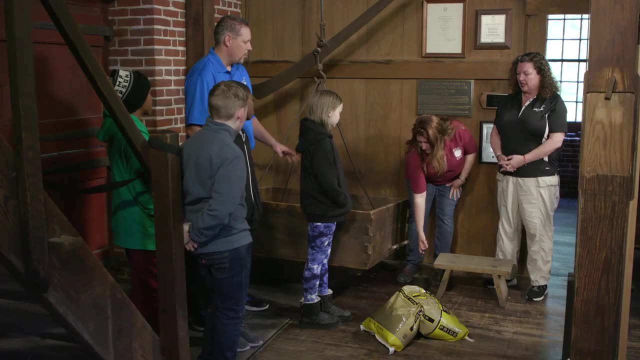 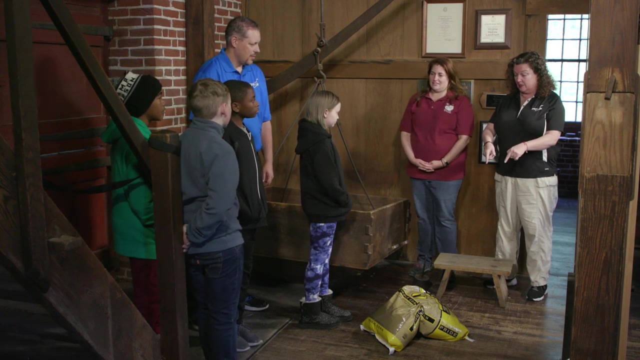 And I can read how many hundreds of pounds of grain that the farmer has brought, And this scale here can weigh about 900 pounds of wheat. Well, let's see how the lever works and how much easier or harder it is for Claire to lift this bag of corn. 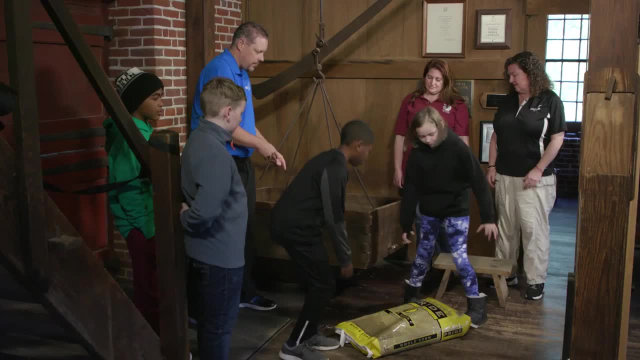 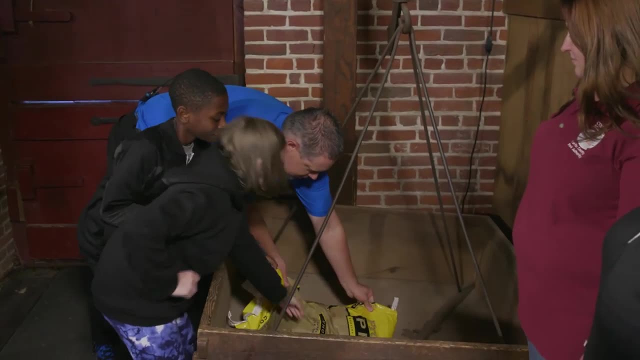 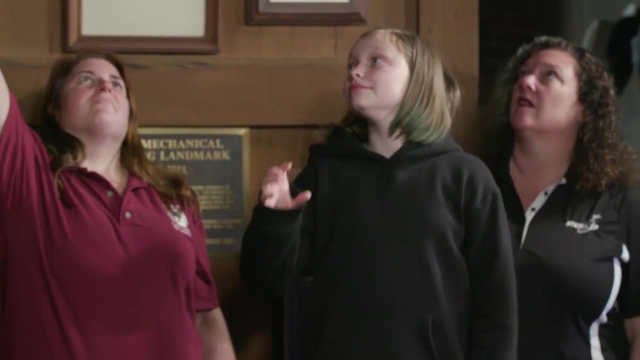 All right, why don't you all grab the bag of corn and let's put it in here, Bring it back over here. Good job. Now, Claire, let's send you over there and see if you can pick this up a little easier than when you were just trying to pick it up off the ground. 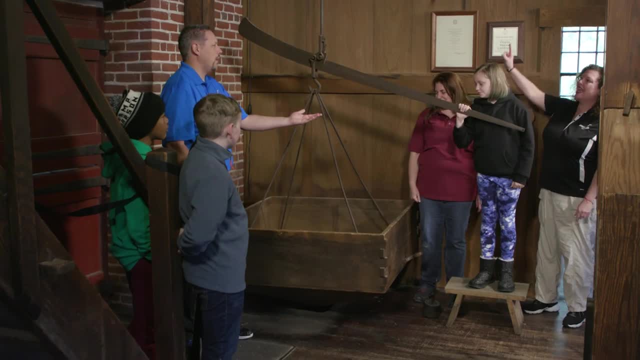 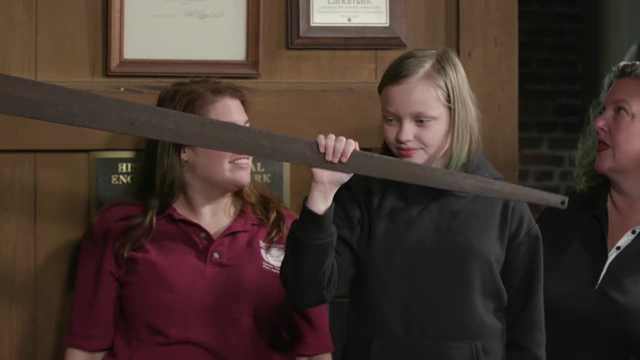 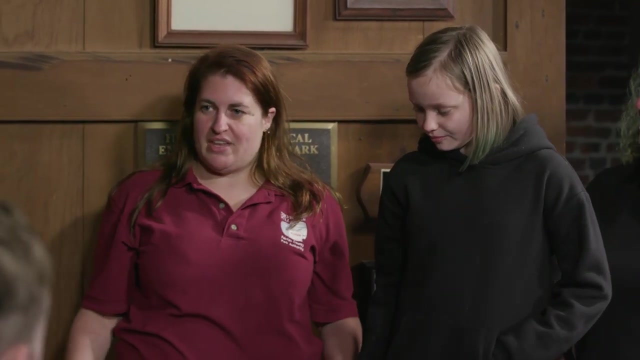 Wait a minute. you're lifting that up with one hand. What's going on? Lighter, Lighter. It's much easier, Catherine, do you want to tell us why this is working this way? So a lever is a simple machine that's used to push, pull or lift a load. 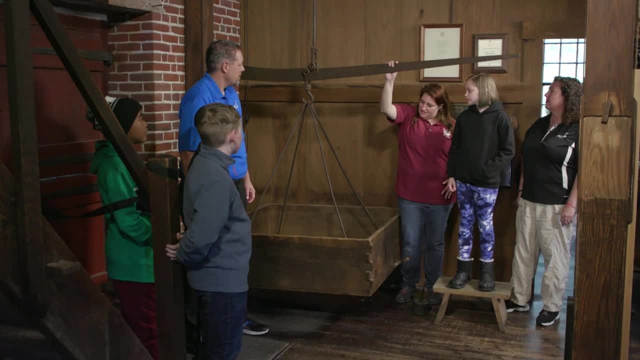 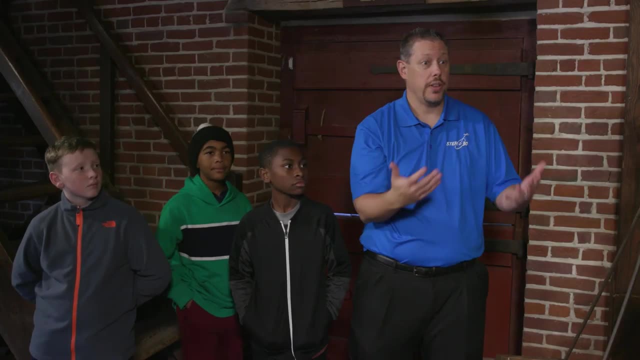 So this lever is pulling that 50-pound bag of grain up and it makes your work easier, And it does that because you've covered it. You've covered more distance with less force. Catherine, this isn't the only lever in the mill. 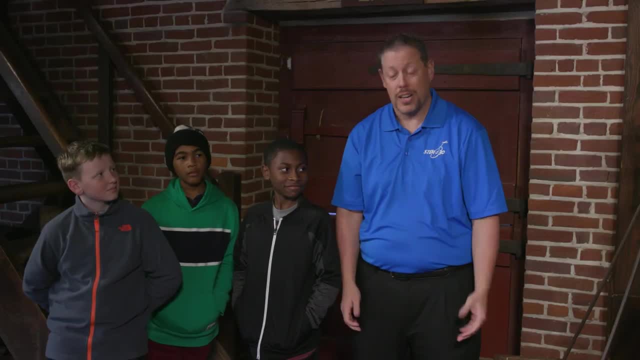 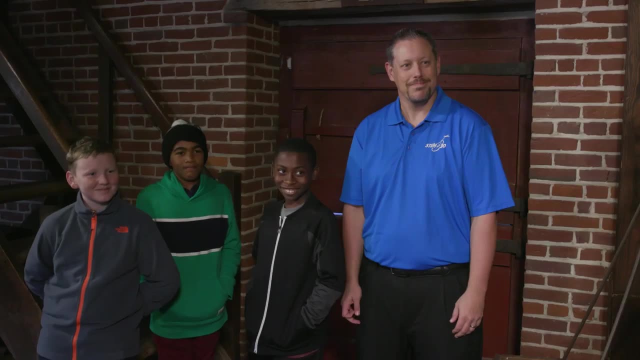 There's a lot of working levers. That's correct. You know, I used to have a dog that I wanted to name Lever- That's a dumb name. My brother decided we should name it Nate, because you know better Nate than Lever. 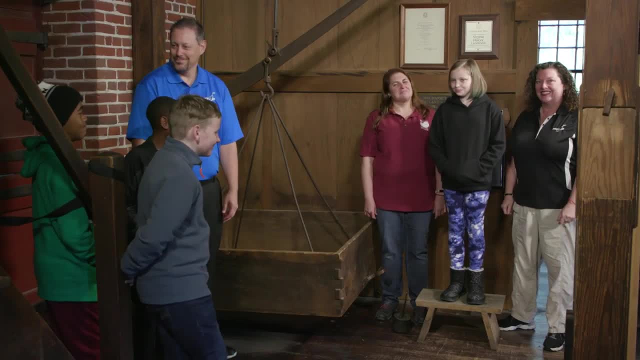 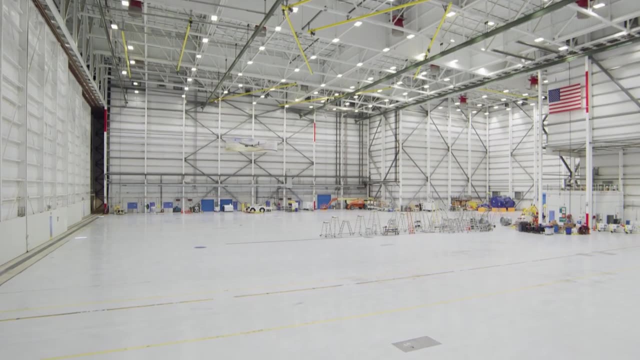 Let's take a look at some modern day levers and how they're used. I am now joined by Brian Kerr and we are in the United Airlines maintenance hangar. We do a lot of high-tech work in here, don't you? Oh, we do a lot of work in here. 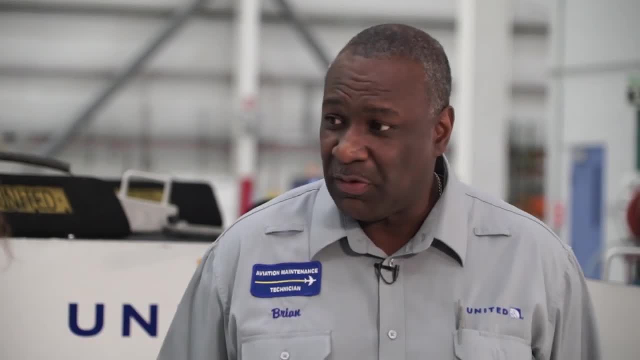 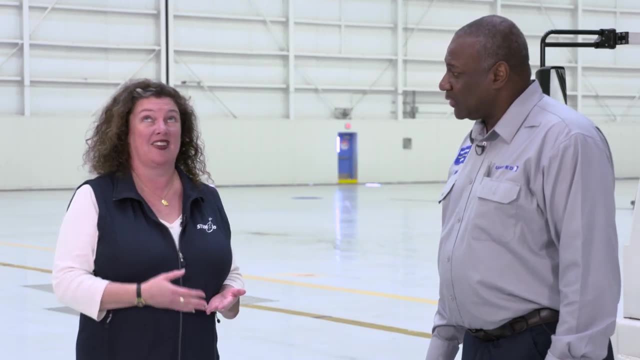 On a nightly basis. we prepare our airplanes for departures in the morning, taking our passengers to wherever their destination may be. And although it's high-tech work, you've got a lot of simple machines in here. I see, for instance, this pulley up here on the ceiling. 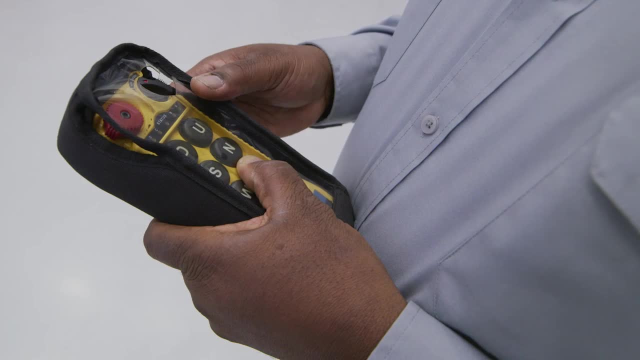 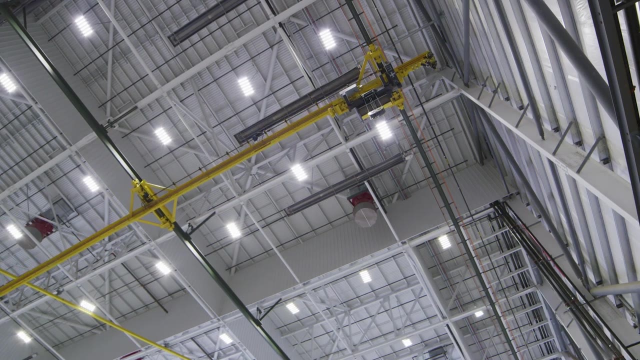 What do you do with this? Well, absolutely, We use this crane mechanism that has a pulley attached to it, And what we do with that is we lift very heavy things. What about levers? Do you use levers? We use levers. 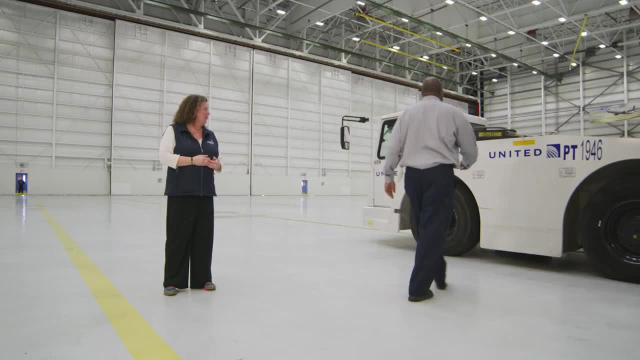 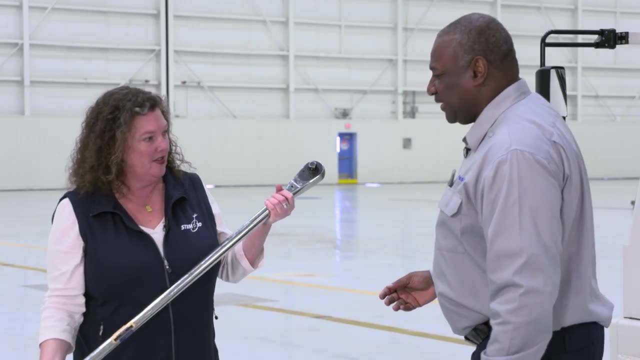 We use levers every single day. For example, we have this lever here which is a torque wrench. Be very careful, It's very heavy. Oh, it is heavy, Yes. So what do you do with this? And we use this lever to torque very high torques on certain things. 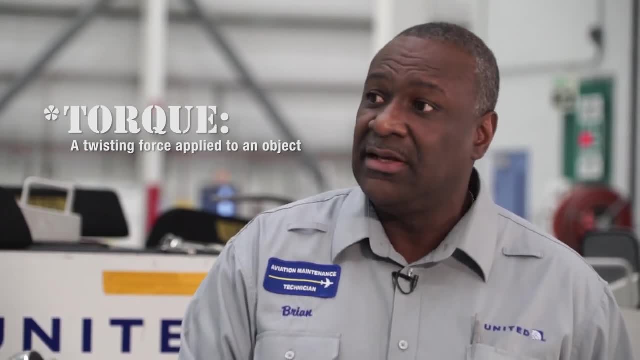 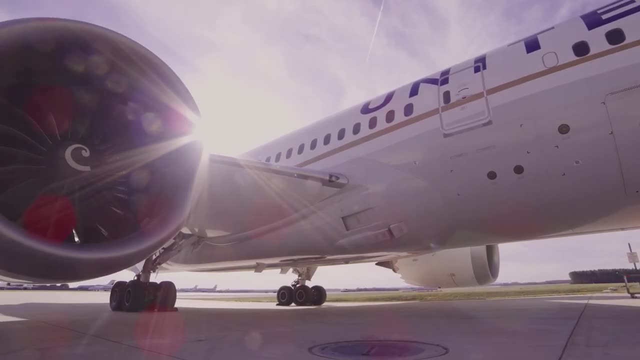 We have certain nuts and certain mechanisms on the airplane that we have to ensure that they're properly torqued. By torqued I mean tightened so that they will not come off in flight. Okay, And one person couldn't do it with a small lever. 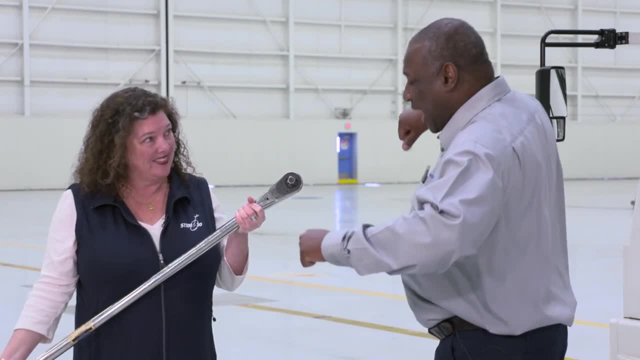 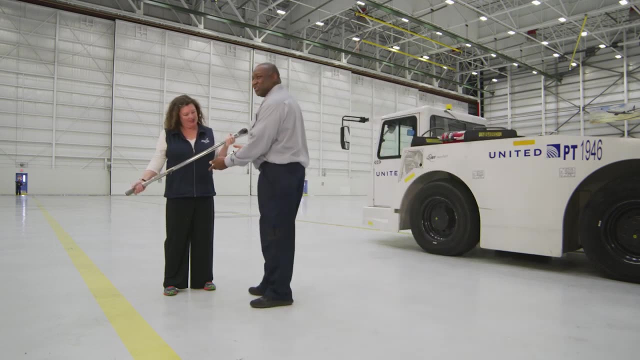 With this one here. sometimes we need two guys on it, you know, actually putting pressure on the lever We also have here, which is another lever, which is pretty much this is a personal lever. Okay, It does the same exact thing. however, one person can use this. 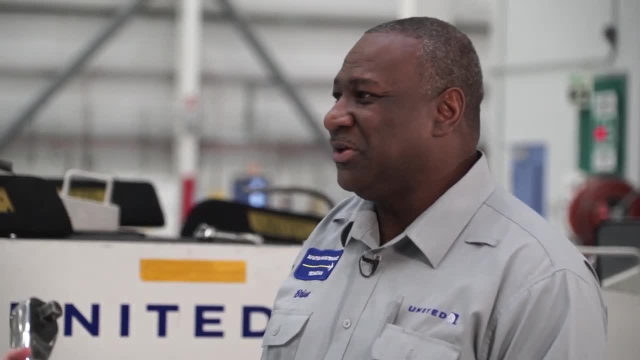 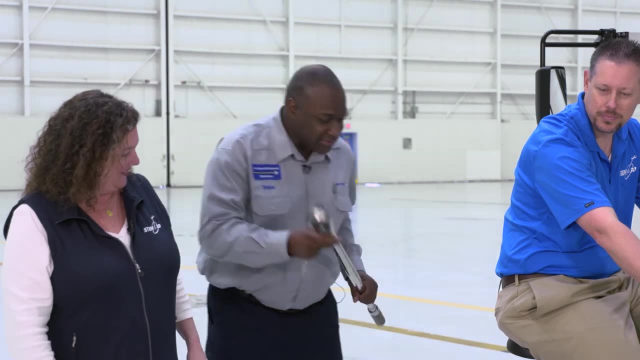 And I saw one other simple machine in here. Well, we have another simple machine that we use every day in here: Wheels, pedals, And what we do we use this for? Okay, It's to transport our technicians around and also to carry things. so he or she does. 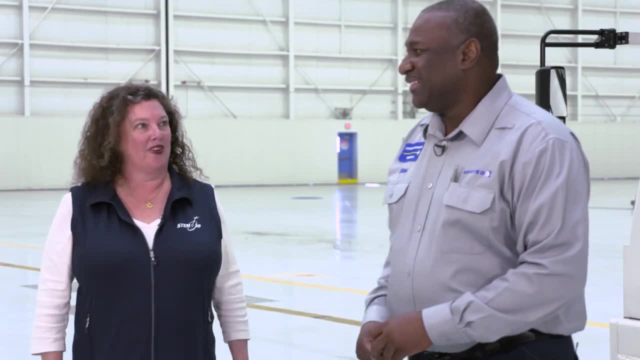 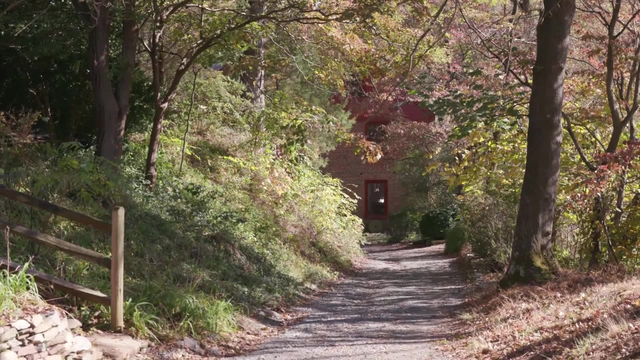 not have to carry them. He's got his wheels and his there. he goes off on his bike. Thank you so much for talking with us today, Brian. You're very welcome. We've moved from the mill to the education center where we are looking at some more simple 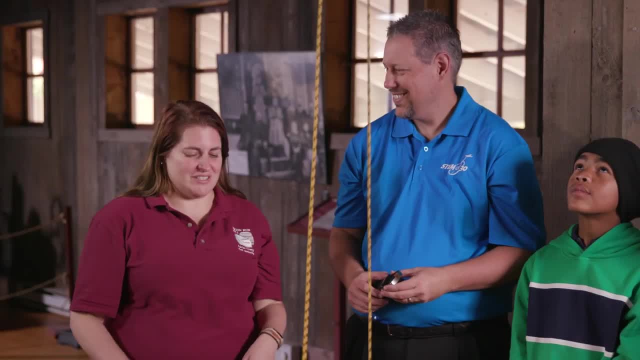 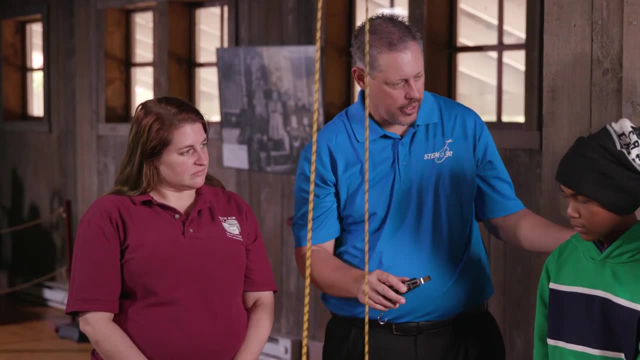 machines. Katherine, what are we looking at here? We have two sets of pulleys. We have a movable pulley and a stationary pulley, All right, So we've got a bag filled with some rocks down here. You look like you're a strong guy, so I want you to take our scale and pick that bag up. 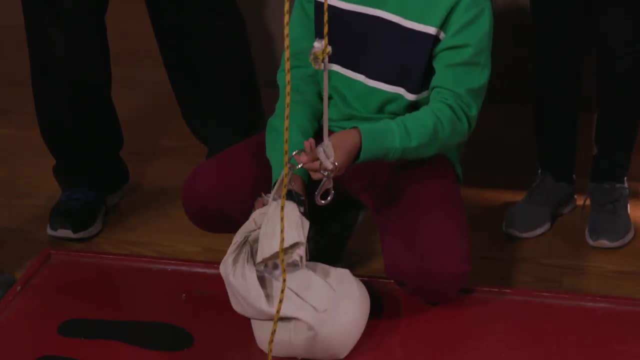 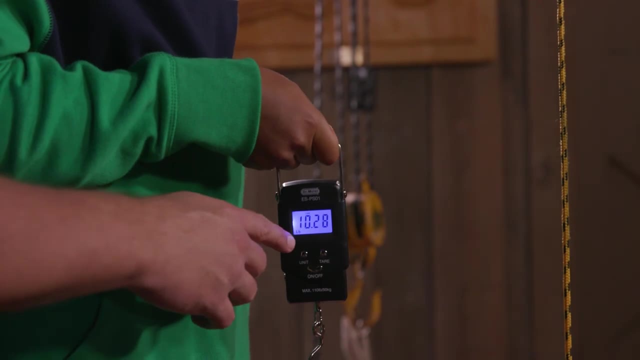 and tell us how much it weighs. Pick that up, All right. What do we got there? That's right about 10 pounds, isn't it? Mm-hmm? All right, Put it down. Okay, Now take your scale off and you hook that bag up for me. 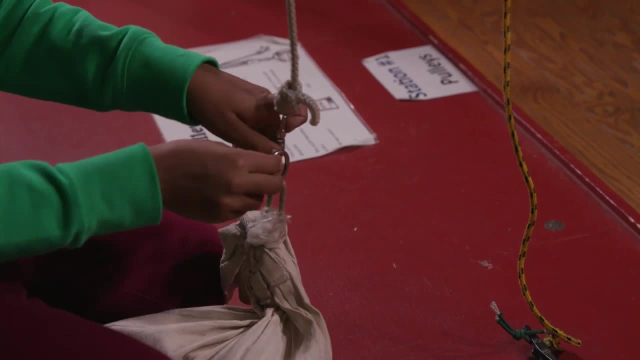 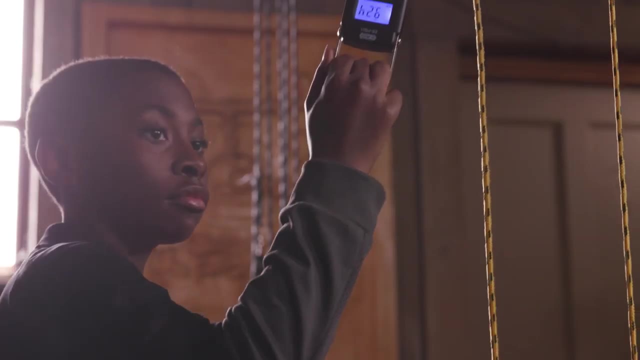 I'll take your scale. I'm going to hook the scale up here. You're going to give this a pull now. Okay, So you give that a pull And let's look and see what the readout says. That's just about 10 pounds, isn't it? 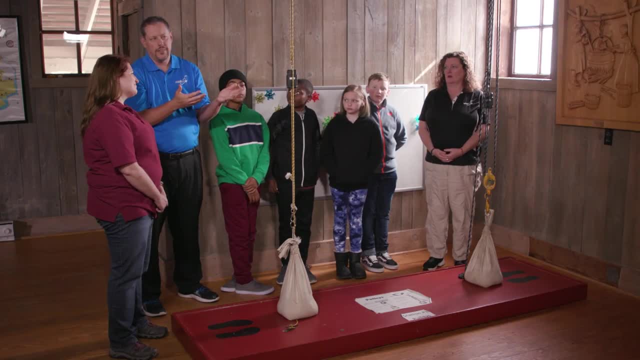 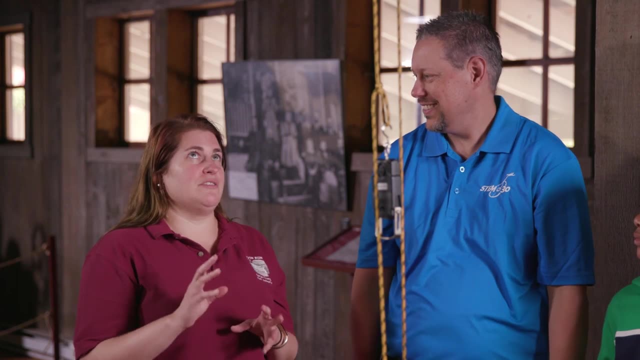 So the same amount of force? Now, Katherine, I thought pulleys were supposed to make our lives easier and that took the same amount of force to pick the bag up as it did using the pulley. What's going on? So all we're doing here with the fixed pulley is changing the direction of the force. 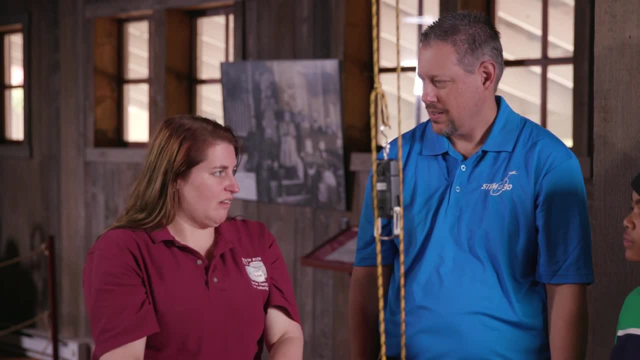 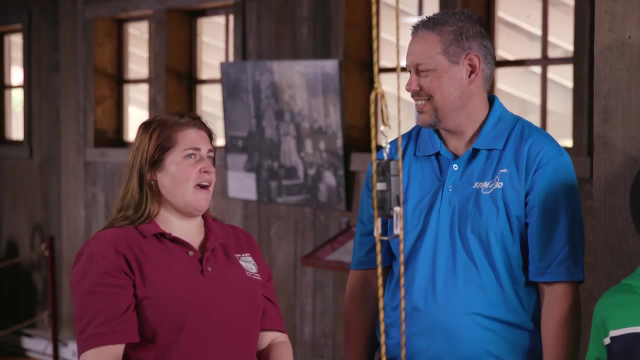 The pulley's staying in place and you're still pulling a 10-pound bag up. And the same distance, All right, But over there it's not going to take as much force, is it Correct? We have a longer distance. 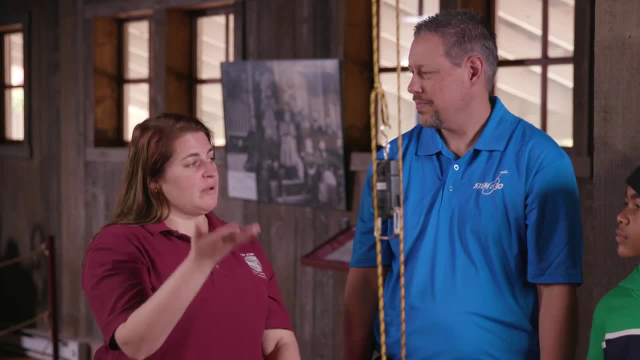 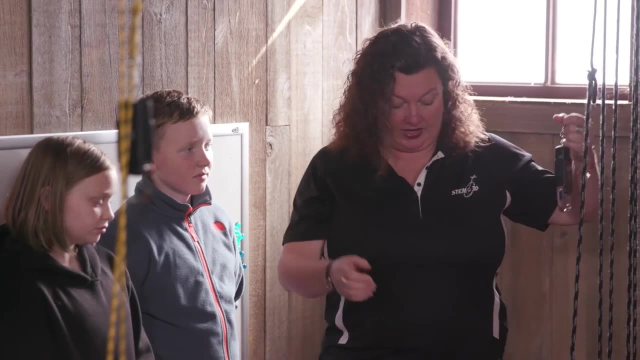 We're using four different pulleys. One of those is a movable pulley that's going with that load. Let's see what happens when we add more pulleys. Come around here. We'll take the scale. We're going to do the same thing that we did over there. 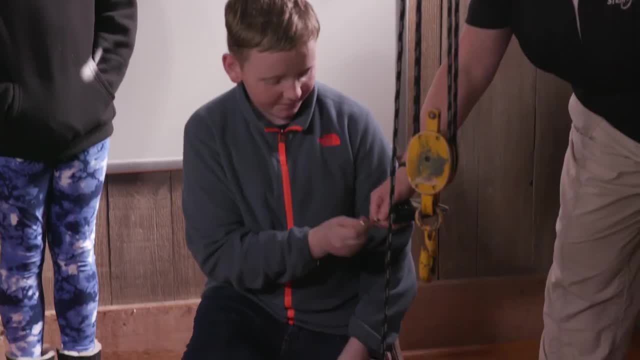 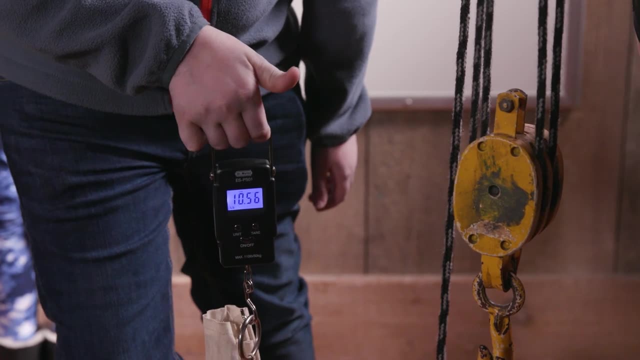 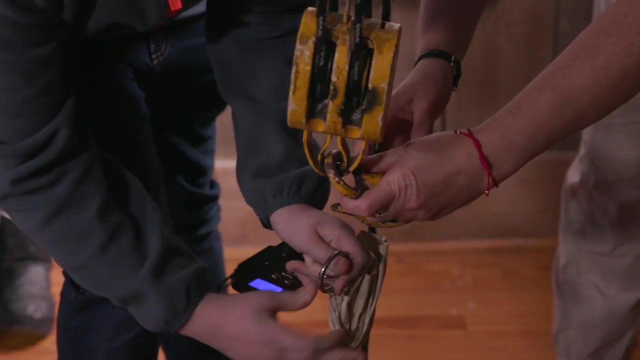 What I want you to do is hook that onto the bag and then you're going to lift that up. We've got about 10 pounds right there. Okay, Put it down Now. Okay, All right, I'm going to take the same scale. 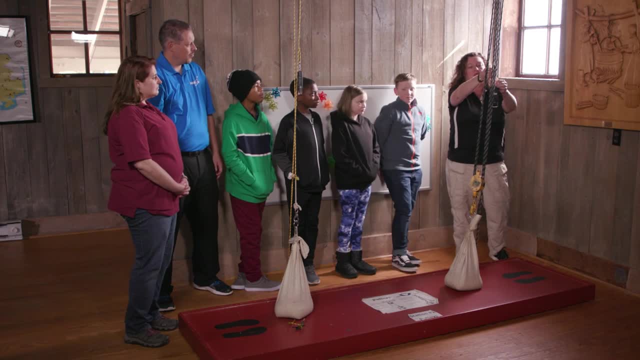 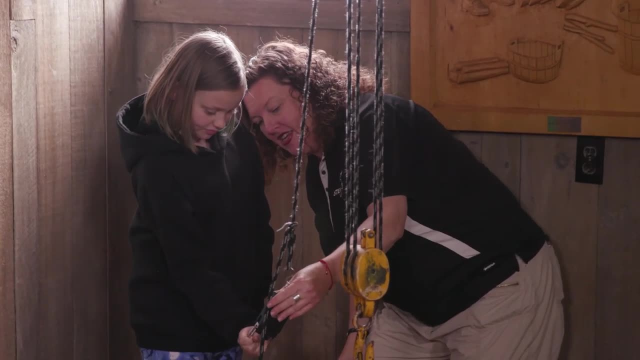 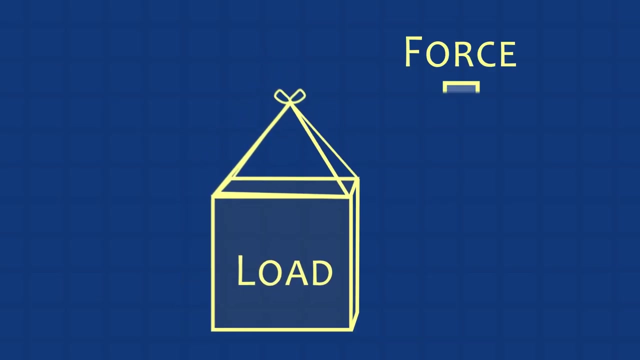 Claire, come on over. All right, You did it with one arm again, and that is a lot less force to lift the same 10-pound bag. What's going on? So what we've done is we've distributed that force over a longer distance, which makes 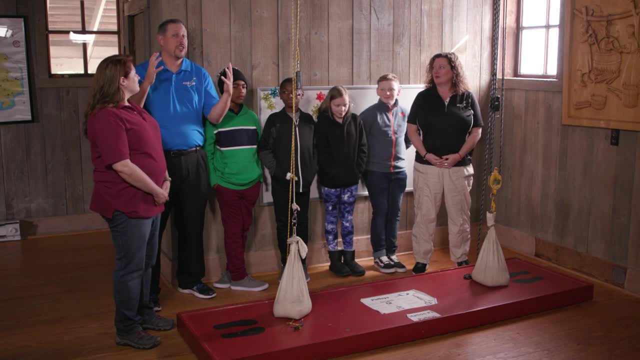 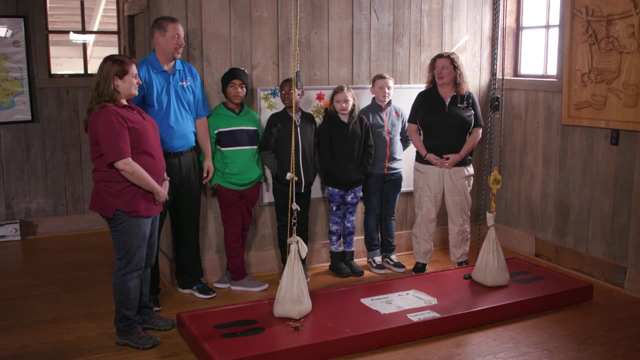 it easier to lift the same amount of weight. Right now, the National Air and Space Museum is going through a lot of renovations and there are a lot of ups and downs involved with that, including some using pulleys. Let's take a look at how we're using pulleys during renovation at the National Air and 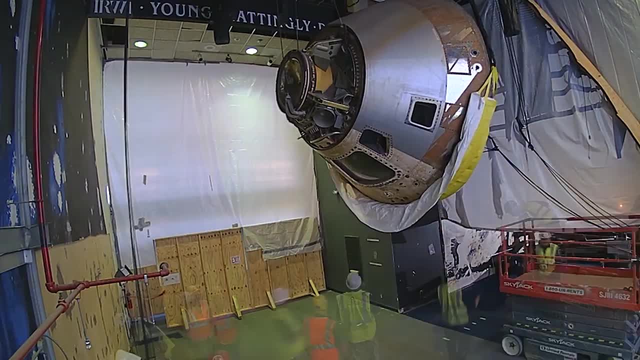 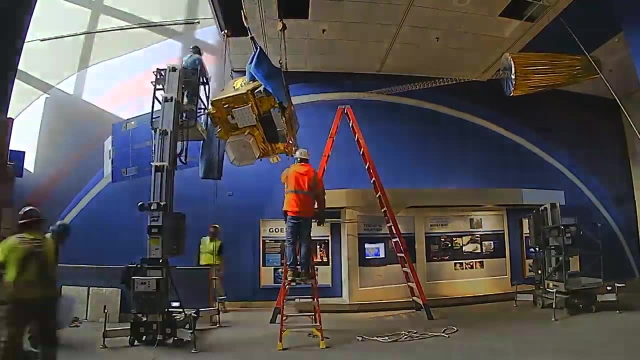 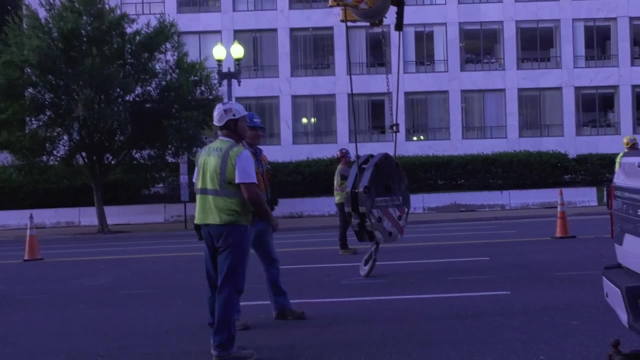 Space Museum. Large airplanes and spacecraft need to be moved during the museum's renovation, as well as really heavy construction materials, Some of these objects weighing thousands of pounds. Many simple machines are used to accomplish this. Often, these simple machines are combined into complexity. 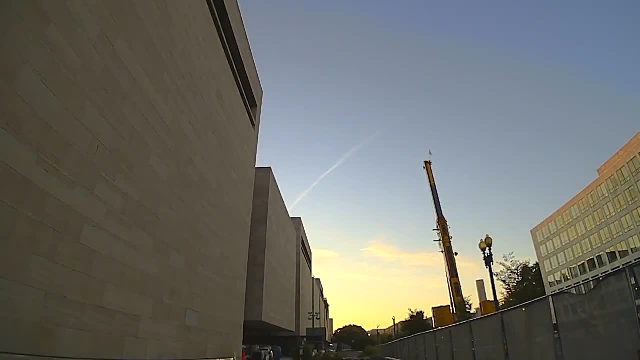 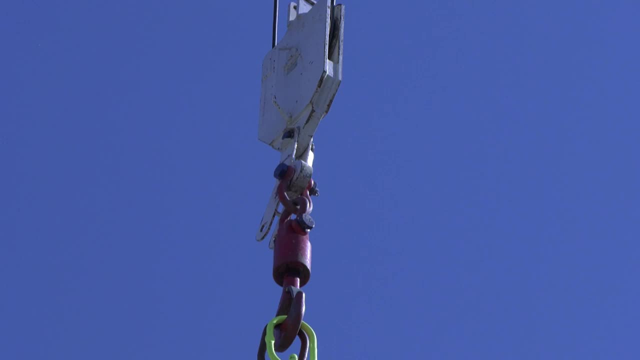 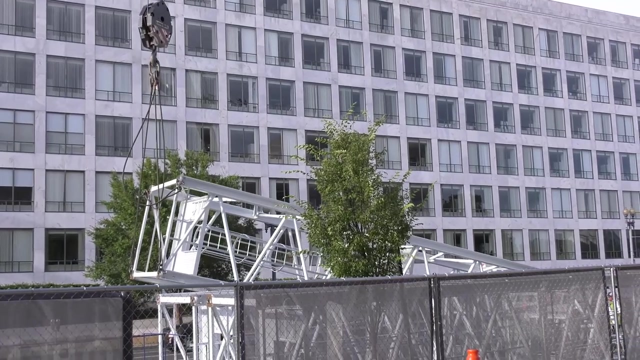 They are combined into complex machines to accomplish these enormous tasks. To raise and lower large objects, pulleys are used. A pulley itself is a wheel and axle that changes the direction of the force applied. With a pulley, pulling down makes something go up. 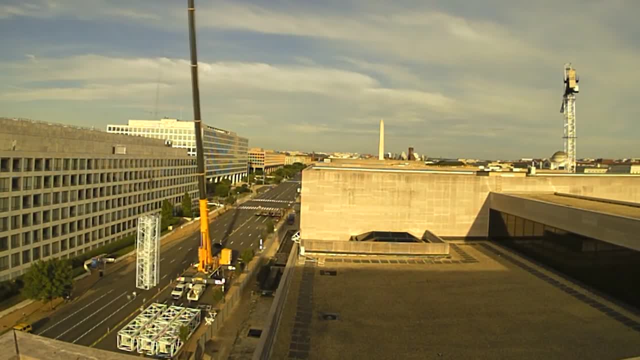 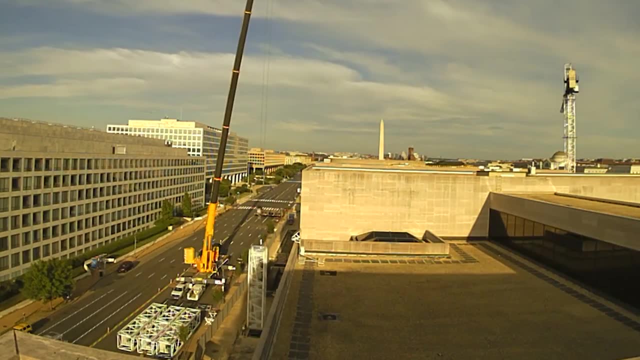 An object called a load is on one end of the pulley, and when enough force is applied to the other end, the load rises. Pulleys can also be combined to create a mechanical advantage. Allowing your machine to move is a great advantage. 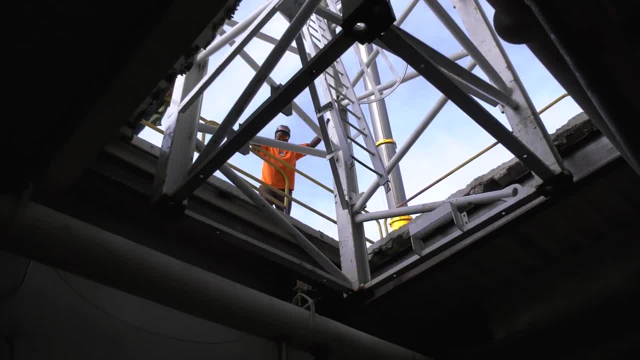 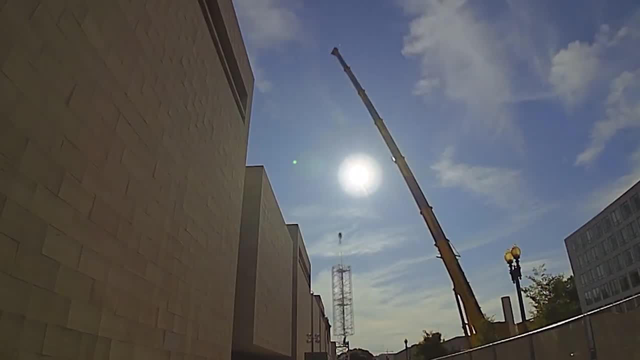 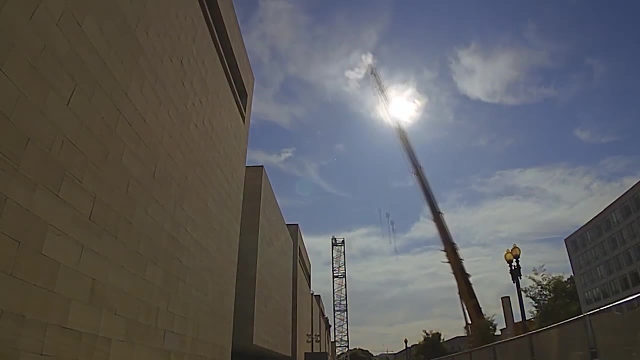 It allows you to amplify the effectiveness of the force you applied For a pulley. this means pulling a longer distance but using less force. A crane is a complex machine that uses mechanics to carry heavier loads than humans can. It combines many simple machines like the wheel and axle and levers. 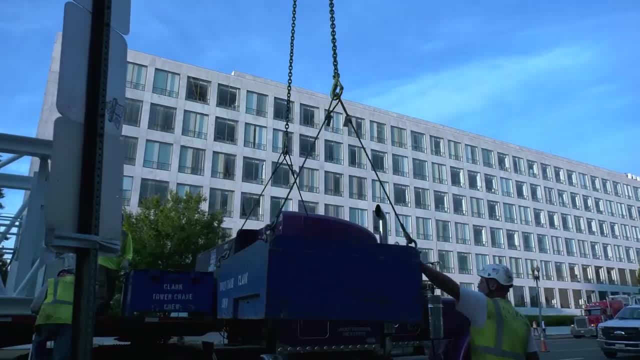 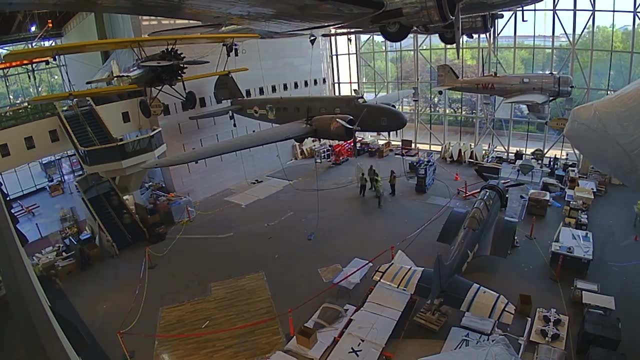 A crane uses a wheel and axle to move loads rotationally, but one of the most noticeable are the pulleys suspended from a projecting arm and used to move really heavy objects vertically as well. All of the artifacts come down and need to be moved out of the museum.